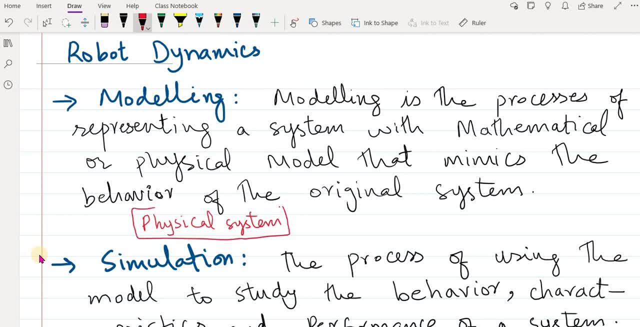 and so what you are going to do is you represent a system in, in the form of mathematical equations, though this is called. so this process is called Ayurvedic plot, called modeling. so, for example, you have a robot, okay, um. so one way is you have a physical robot and you actually perform. 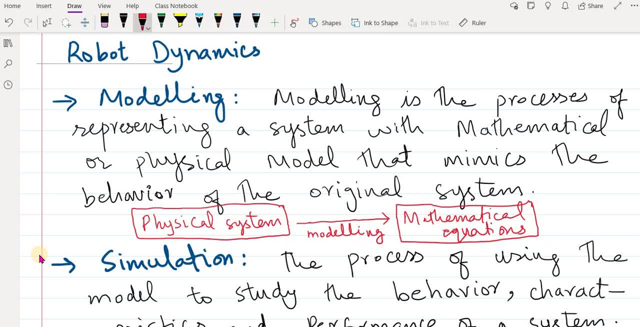 kinematics on this robot. okay, you, you, you enter some values on its microcontroller and then run the code and then the robots move to a certain position according to your joint angles. the second way is you, you make a model of this system, of this robot. you know, you have now mathematical equations. 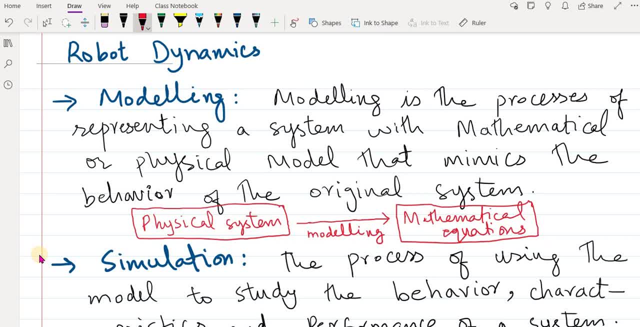 and then you give input to this mathematical equation and then you get output which which is same as the physical system. so this is an advantage of using a physical- sorry, using a mathematical module. you can model anything using mathematical equations. you can model a car, an aeroplane, a robot using mathematical equations. so the advantage is that you 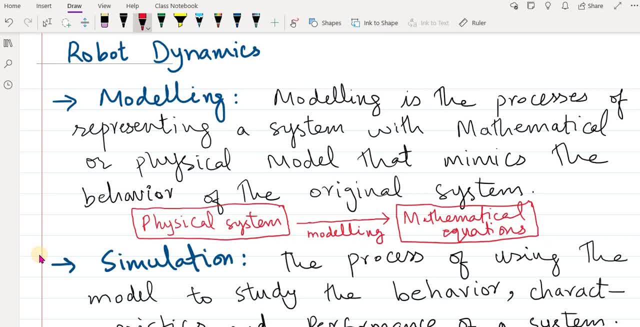 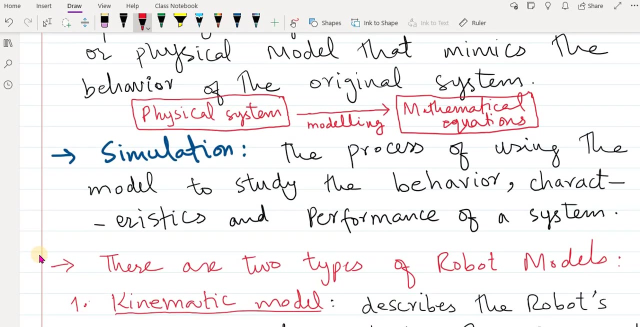 don't need to purchase or buy actually an aeroplane or a robot. you can just make its model and you can predict its behavior. and if you give this angle, what will be the output position? okay, so this is the. this process is called modeling. now, what is simulation? the process of using the model. 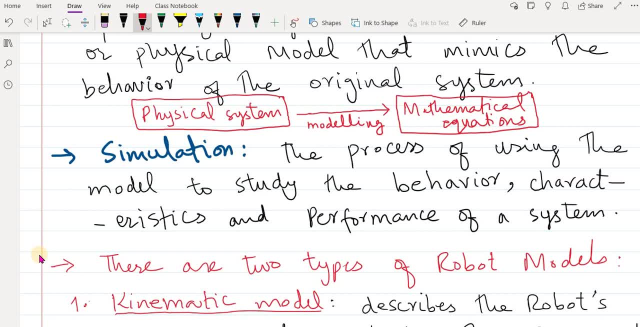 to study the behavior, characteristics and performance of a system is called simulation. so once you have a mathematical model of robot, so then you give some inputs to this model and then you get some outputs. for example you get joint angle and you get the position of the and effective of the robotic. 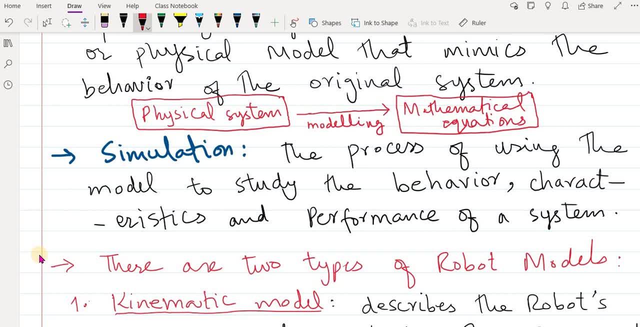 manipulator and then you can. now you see that you are actually mimicking the original physical robot using the mathematical model and you are also studying its behavior, its characteristics and also the performance parameters. so this process of mimicking the original physical system or a robot is called simulation. 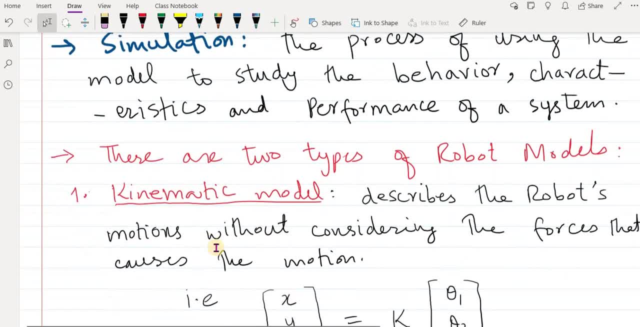 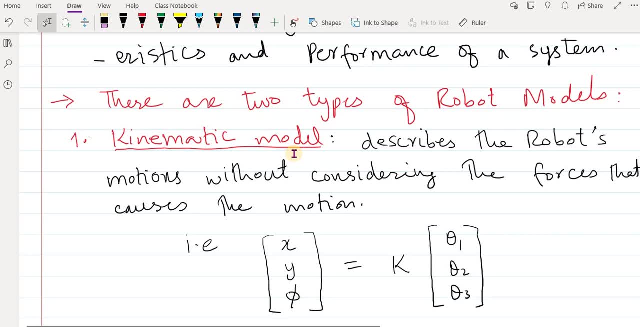 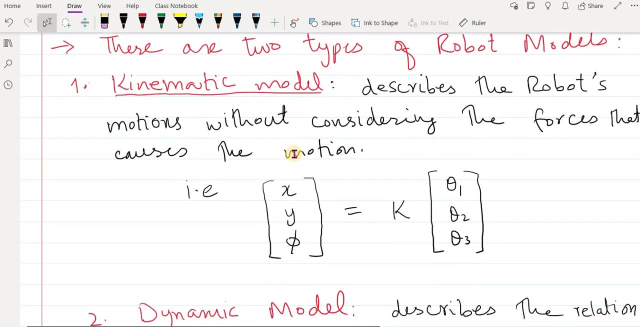 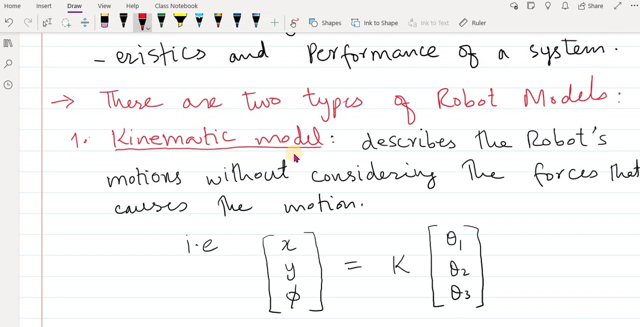 There are two types of robot models. The one we already studied is a kinematic model. In the previous lecture we talked about how we can model a robot using a kinematic model. So what is a kinematic model? Describes the robot's motion without considering the forces that causing the motion. 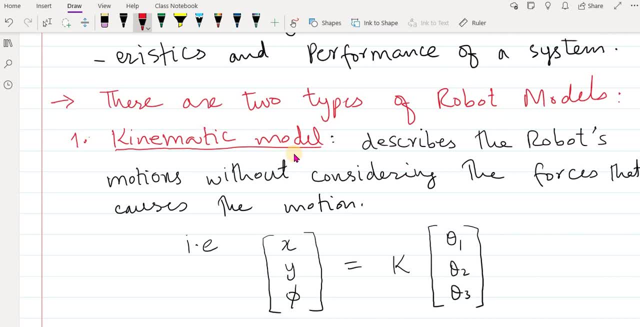 So what is a kinematic model? Describes the robot's motion without considering the forces that causing the motion. So what is a kinematic model? So what we here in a kinematic model, What we are interested in, only the position, either linear position or angular position. 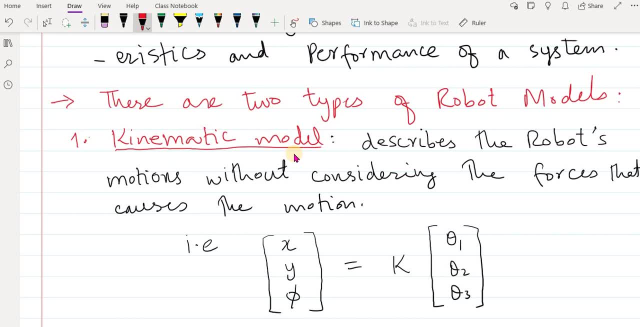 So we know the joint angles, the angular positions of the joint, And we have some function that transform these angles into the position and orientation of your end factor. Notice that there are no forces involved here, Just only the motions or the positions. So these types of model is called kinematic model. 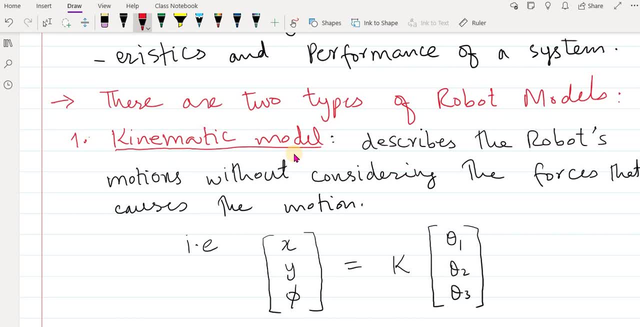 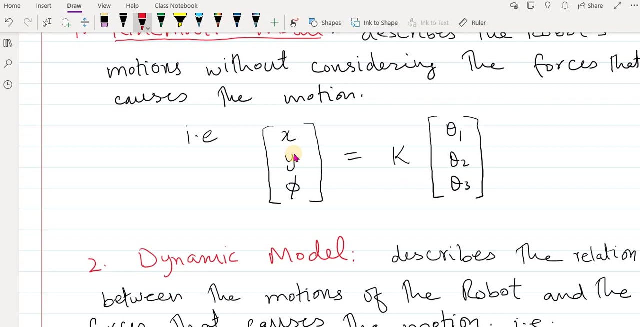 So this is this equation. It shows a kinematic model of a robot. You don't need to actually buy a robot to, Or you have to To find the relationship between the joint angle and the position of your end factor. You just need this equation, Where k is a function that can transform these angles into the position and orientation of the end factor. 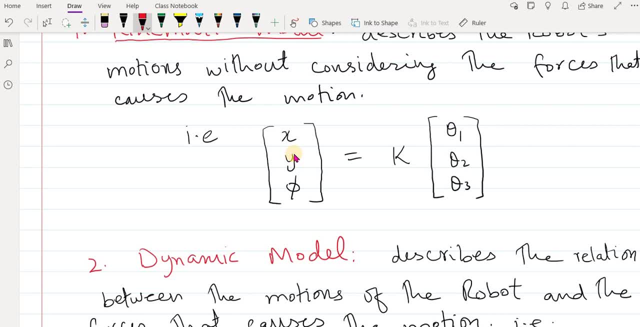 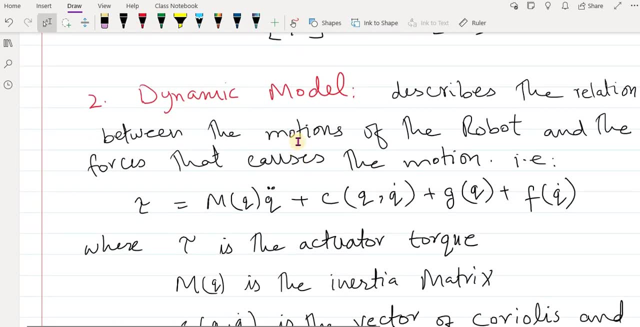 To find the value of k: Just see the previous lectures. Another type of model is called the dynamic model. A dynamic model describes the relation between the motions of the robot And the forces that causes the motion. So in a dynamic model We also study motion, But in addition to motion. 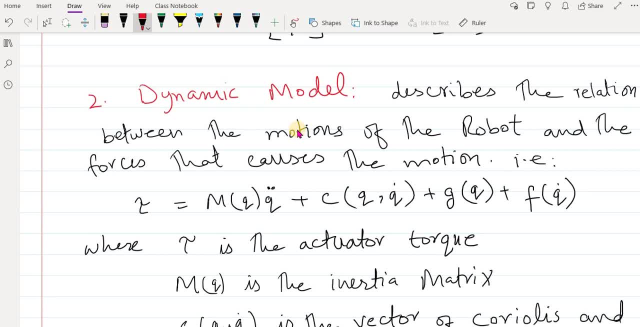 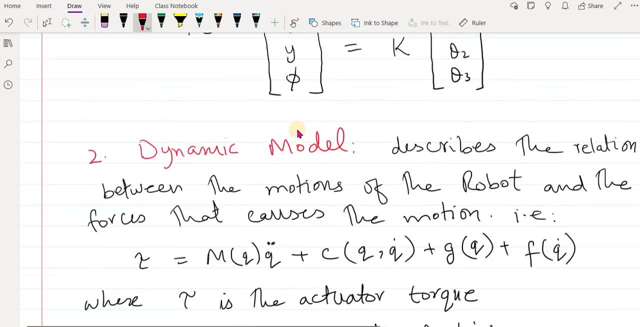 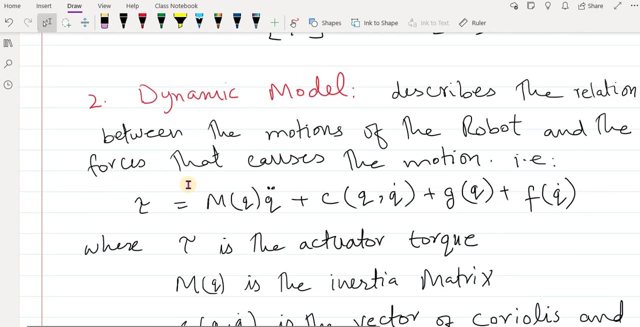 We also need to include the forces, or torques, that causes this motion, And remember that in the kinematic model We just ignore the forces. We were just concerned about the motion, But here we have to study the torque or the forces. For example, A dynamic model might look like this: 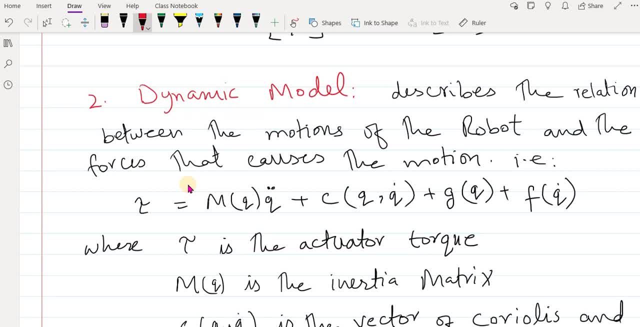 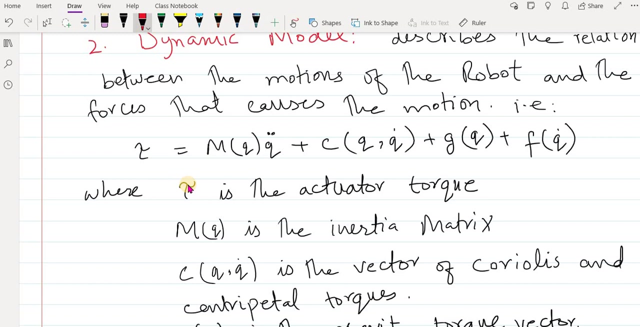 Where the Your applied torque or applied force Is equal to the, The inertia, Inertia of your system, Where m is the inertia matrix and q double dot is the Either linear acceleration or the angular acceleration, And then you have the These kind of Centripetal torques or forces. 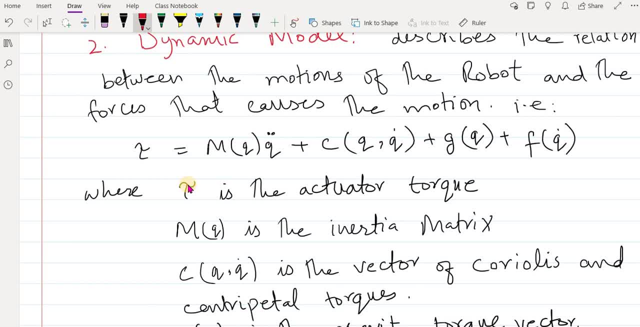 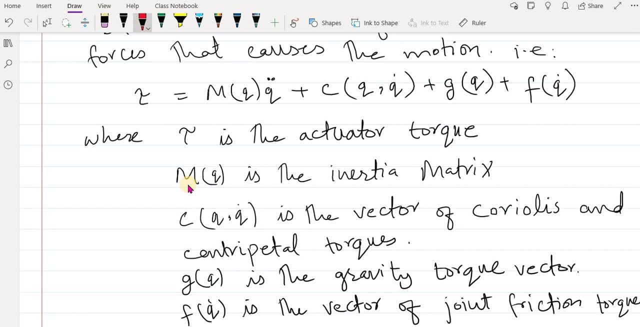 Terms. And then you have some gravity, Gravity, torque vector here- And finally you have some friction, The torque or the forces That causes friction. So just keep in mind that whatever you The torque or the force that you apply to the, The link or the joint of the rope, 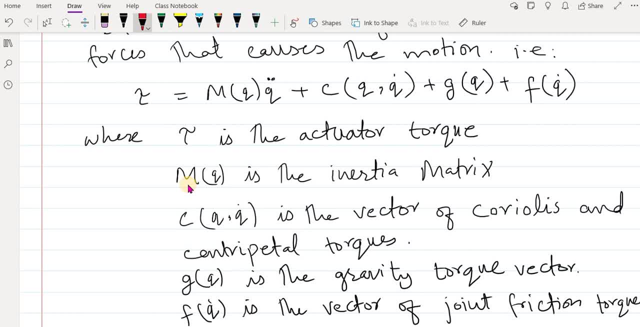 It will eventually Transform into the moment of inertia of the Robot, link Some Centripetal forces And Also work has to be done against gravity And also Some of the your torque will be Dissipated in terms of Friction. So this is the Typical example of how 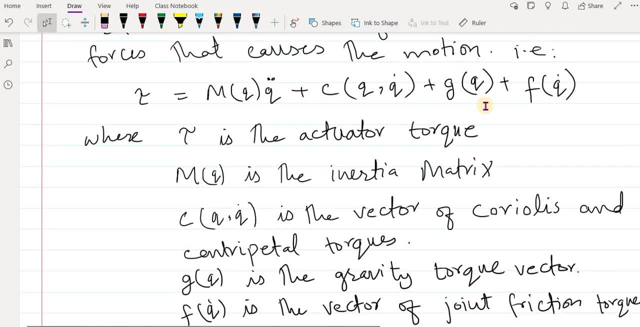 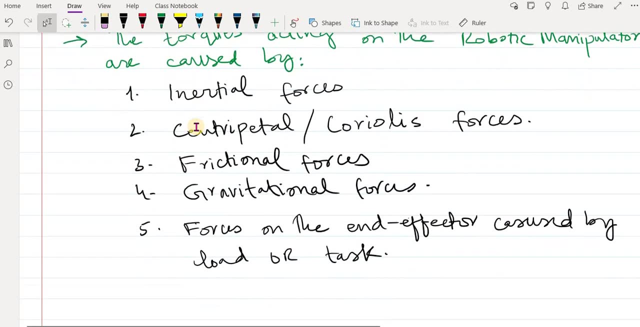 A dynamic equation looks like, Or sometimes we just ignore friction, We ignore some forces, And then this equation will be Simplified further. The torques acting on the robotic manipulator Are caused by. So again here There are different types of torques That are being acted on a robotic arm. 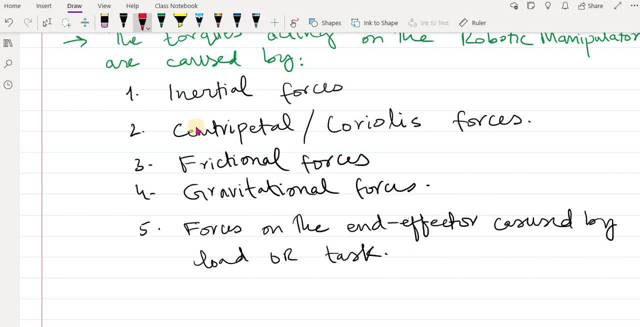 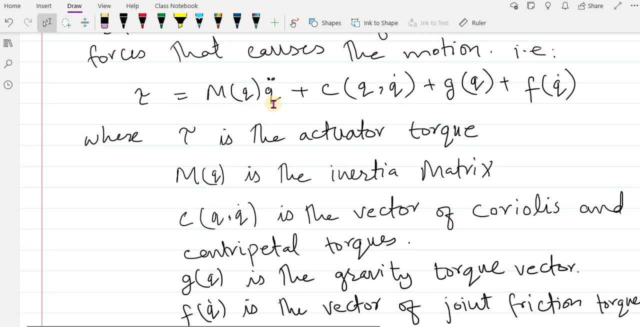 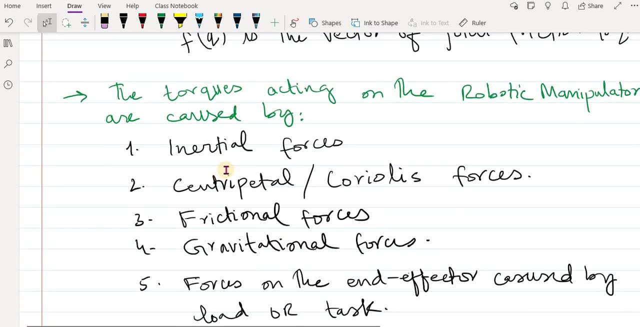 So So The torques can be from Inertial forces That we have mentioned here This M term: MQRR, This is M, This is acceleration into mass, Which is shows that Your applied torque Is converted into Inertial force Or inertial torque. The second type of torque can be: 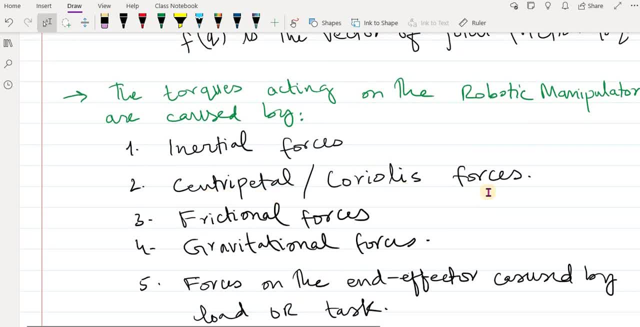 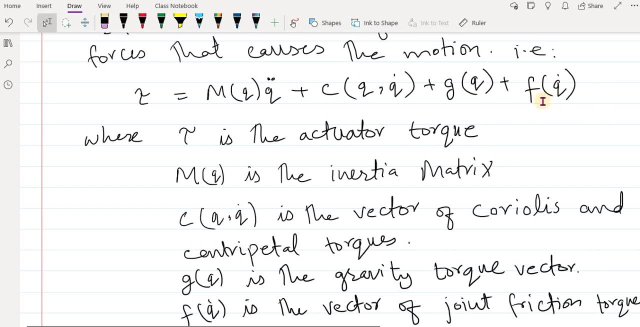 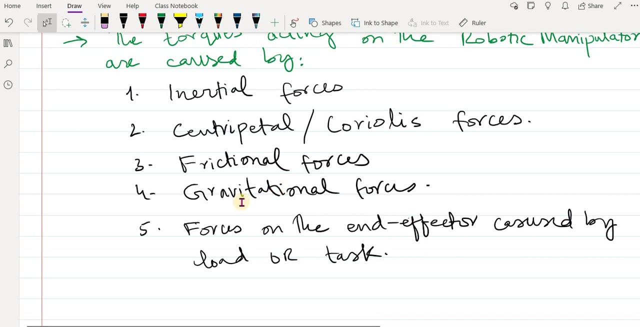 Centripetal or Coriolis forces. Third type of torque can be Caused by Frictional forces. The term here Due to frictional force, Friction between the, The joints. And then the fourth type of torque Can be from Gravitational forces. We shall study later. 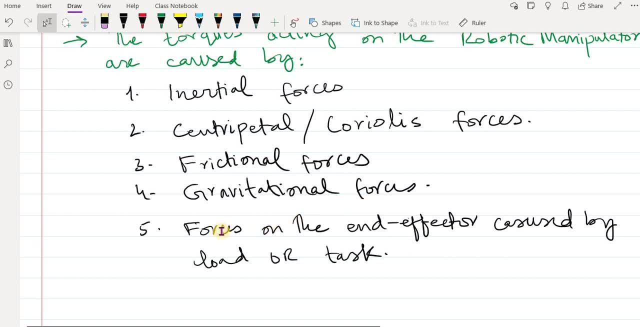 How gravity creates a torque And then forces on the end effector Caused by load or task. So whenever There can be torque Caused by a force Coming from the A load attached to a end effector, So in this case you have to Do a work. 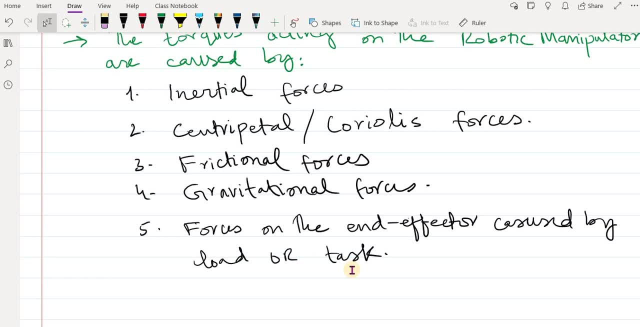 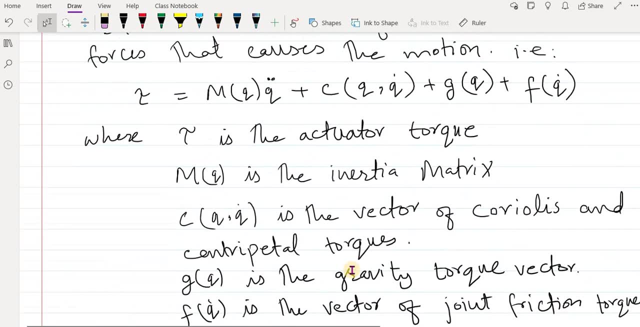 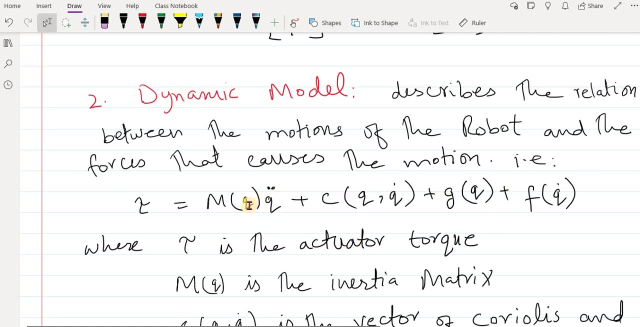 Against this, Lifting this Load. So, Yeah, So these were The torques and forces Found in the Manipulator And together, adding up, They, They sum up to create Torque, Torque, that is That counteracts With your applied torque, Which is Which is coming from motor. 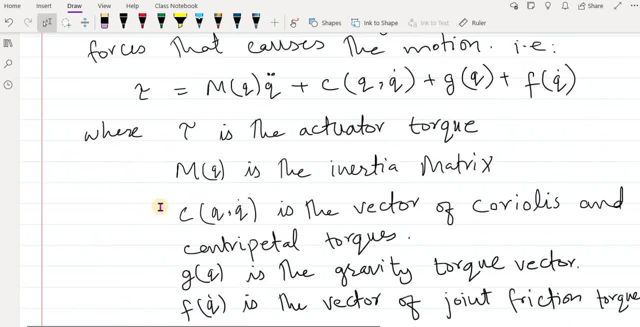 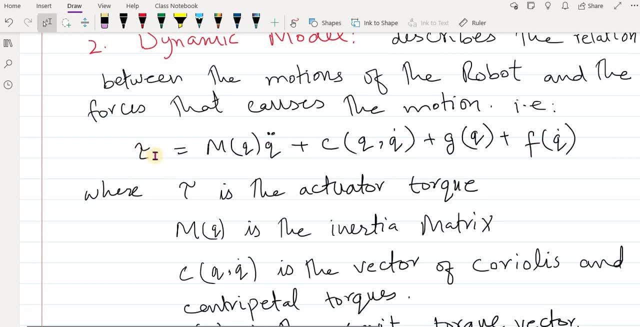 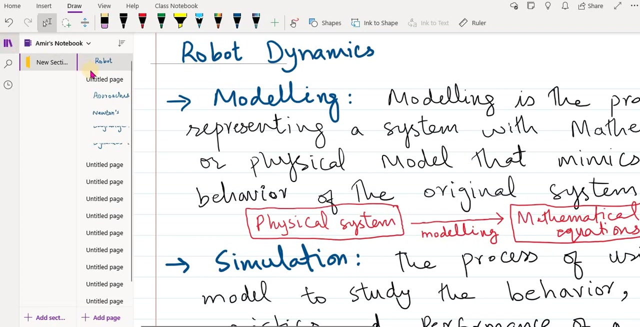 Okay, So this torque, here It's. This is applied, torque, By your motor To the joint of the robot, And then it is dissipated In the form of Inertia, In the form of centripetal forces, In the form of gravitational forces And friction. So now let's move toward the next slide. 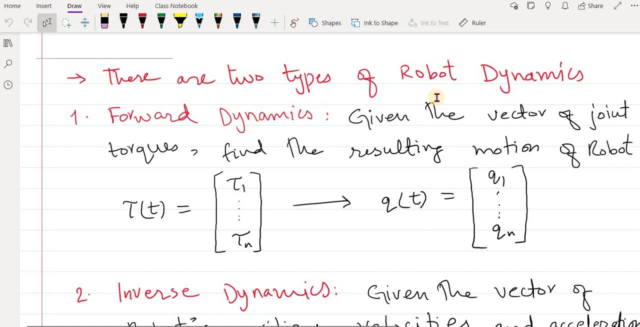 There are two types of robot dynamics, So One is called the forward dynamics And second is inverse dynamics. It seems like we did in Kinematics. we have We had Forward kinematics and inverse kinematics. In forward kinematics, if you remember, We had the Joint angles were given. 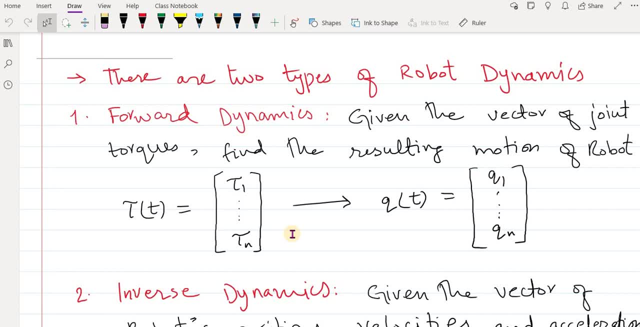 And you have to find the position of your End effector. But in inverse kinematics, You, The position of your End effector was given, But you have to find the position Of your Joints, the angles. So In case of dynamics, We have Forward dynamics And in forward dynamics. 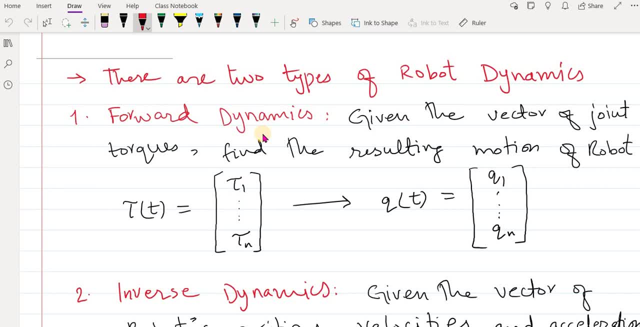 So the vector of joint torques Is given. So you have given, with the torques, Find the resulting motion Of the robot. And so you have to find The, The resulting motion, The, The positions Of the. you can say the, The angles you can. You have to find. 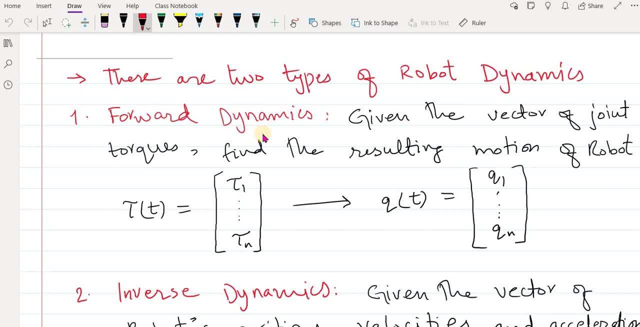 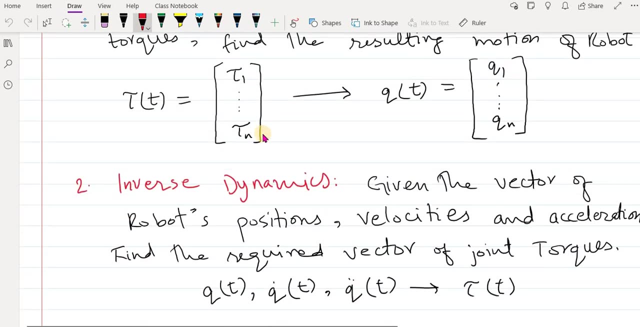 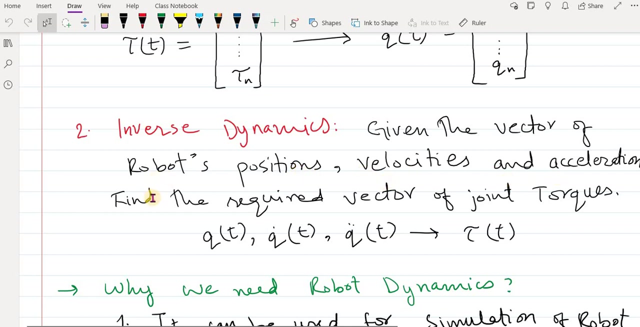 So If this is a one link robot, then The torque is given, How much torque is applied, And Then you have to find the position of the, Of its Joints In inverse dynamics. So the vector of robot's Positions, velocities and Acceleration are given, Find the required. 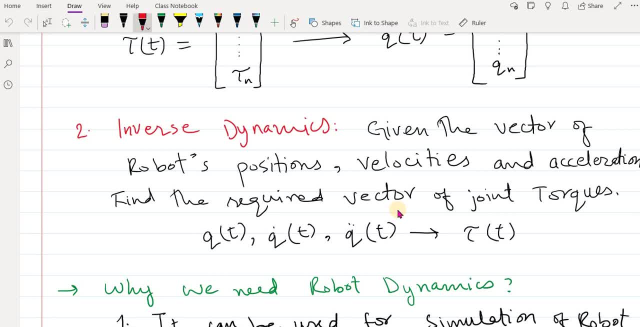 Vector of joint torques. So in this case it is Other way of Drawing around. In this case you have, You are given with the position, Velocities and accelerations And you have to find the Torque. How much Torque must be applied To the joints So that to get? 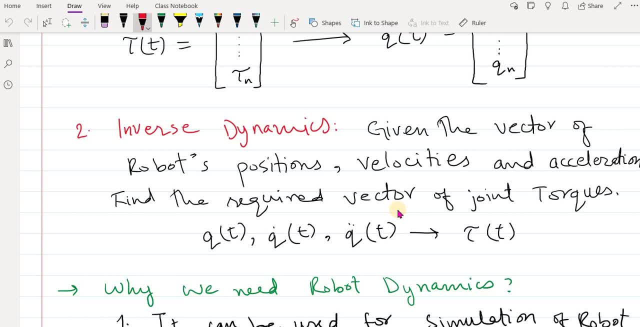 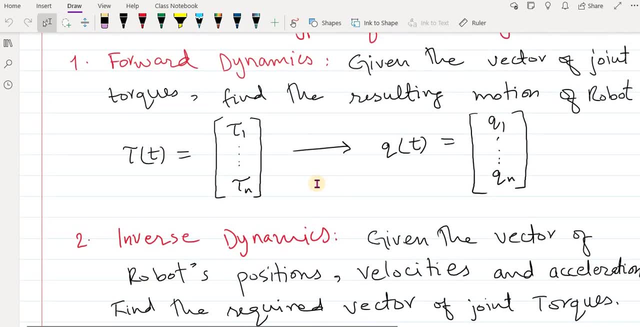 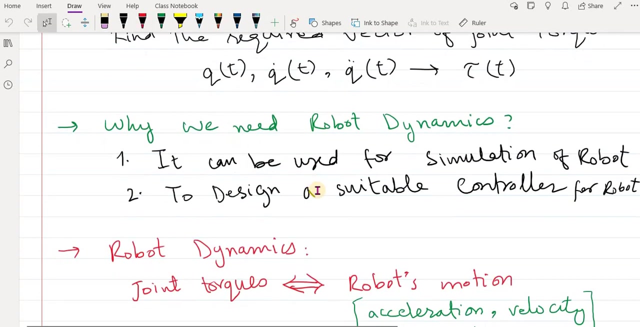 The desired position- Velocity and Acceleration. But in case of forward dynamics It was Other way around: The torque applied was given Okay, And you have to find the position of the joints Or their velocities or their accelerations. Why we need robot dynamics. Actually, You remember that In the previous lecture we talked about 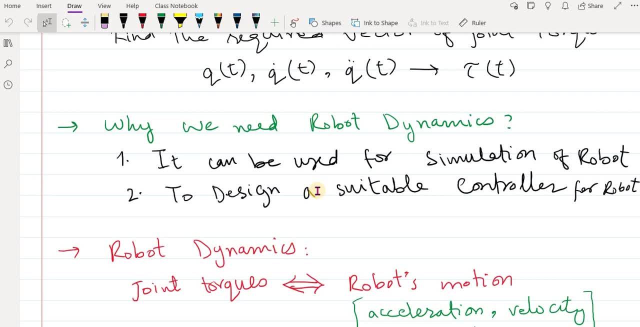 Why we need kinematics. Kinematics was useful For, For example, forward kinematics Was useful for the To, For the simulation of A robotic arm, Okay. and then There was Inverse kinematics, Where you have to find the joint angles, And this case was useful For control of the robot. 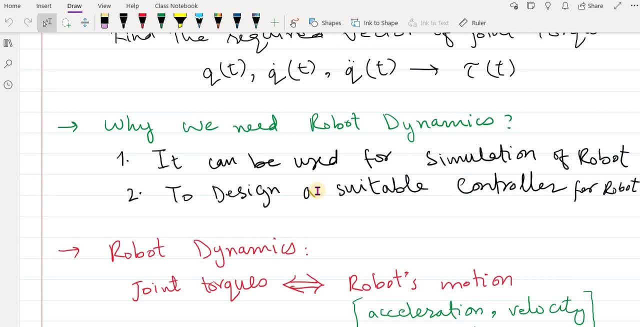 In case of Robot dynamics, The Dynamics is important In the situations. For example, It can be used for simulation of a robot. So when you are Developing with Developing a robot model, There are different types of models We have Depends upon what you are looking for. For example, There can only be a kinematic model. 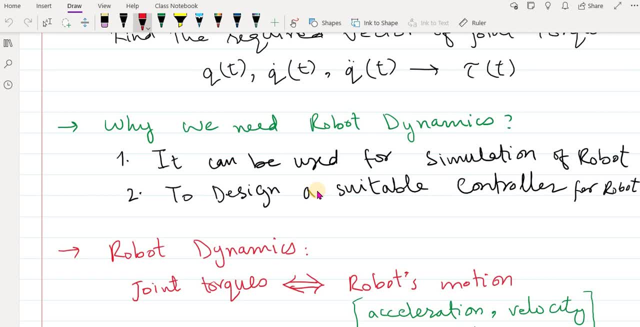 Okay, And then if you want more detail, That your model should look Realistic, According to real world, Then you also have to add some dynamics to it, You have to add a mass, You have to add some Friction, You have to add some Acceleration forces. So 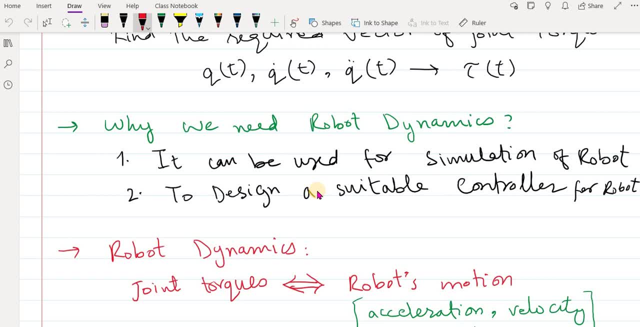 So These all things, They will make your robot Look Closer to the actual Real world robot. Okay, So For simulation It is important, And also to design a suitable Controller for robot. To design a suitable controller, You need to have an accurate Model of the robot If you want to control your robot. 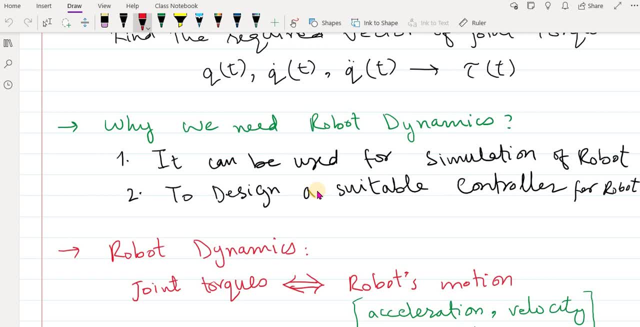 Position, Then you need an accurate controller. For that, You need a more detailed Model of your robot. So That's why robot dynamics is important. We need a dynamic equation Or a dynamic model of the robot, So that we can simulate a robot And control the robot also. So, in short, we can say that: 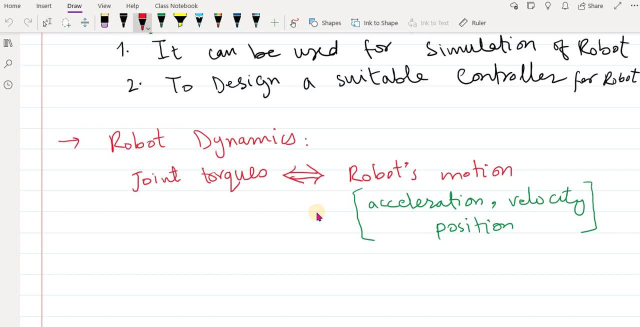 Robot dynamics. What we are doing in robot dynamics Is we have joint Torques Given and we calculate the motion Of the robot, which is acceleration Velocity position. Or we are given Given with the robot's motion, We are given with the Acceleration velocity position And we want to calculate. 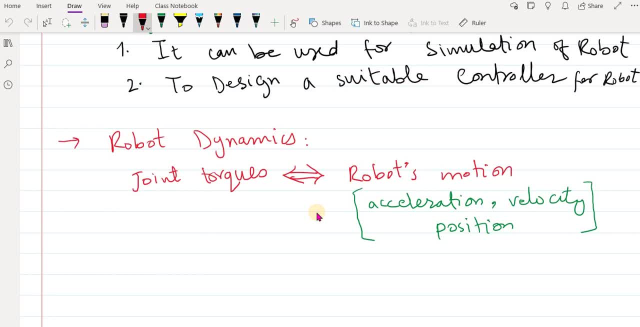 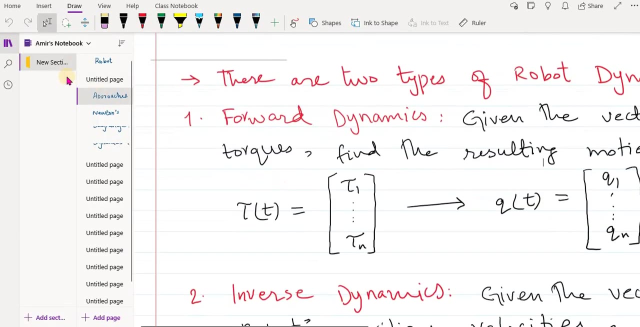 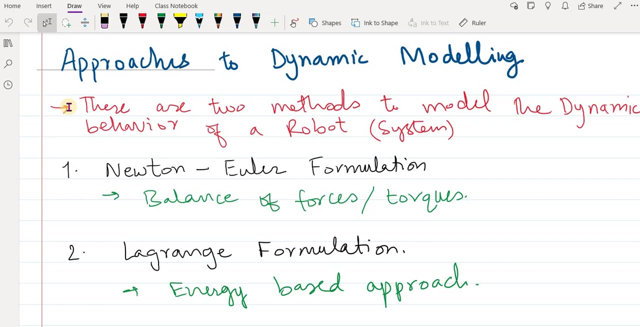 The joint torques. And this thing we cannot do using Only Kinematic model. We must need a dynamic model Of the robot. Now let's see how we can model A robot, That we include It's dynamics, How we can make a dynamic model of the robot. So, basically, there are two methods. 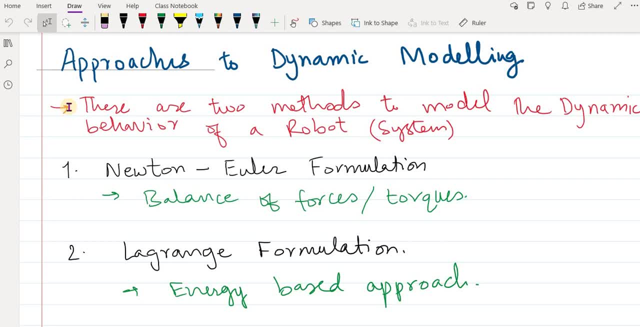 To model the dynamic behavior Of a robot or any system. The first Approach is called Newton Euler formulation. So this Approach is used To basically use Newton's equation Of motions. you can say So. it uses Newton's Equations Of motions And What it does? It tries to balance. 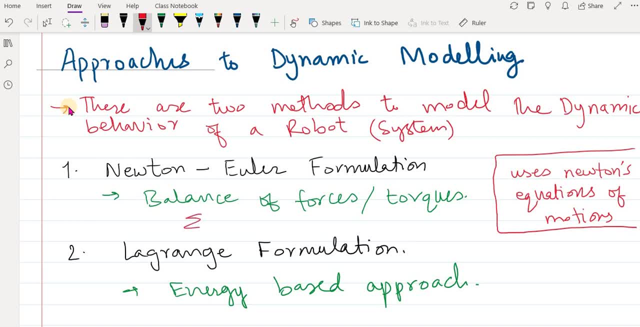 All the forces and torques. And it says that Sum of all the forces Either equal to Zero, or You can say The applied forces are Equal to the dissipated forces, Or you can also say Sum of all the torques is equal to zero. So this is the Newton method. 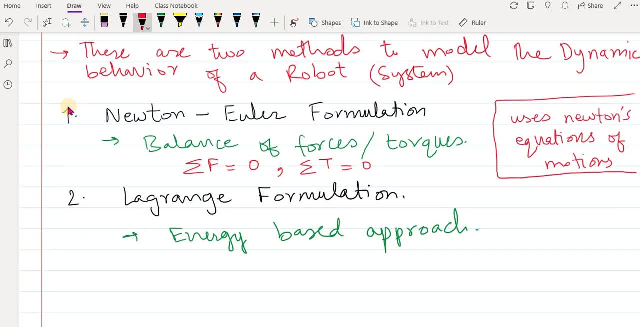 And then There is another method. It's called Lagrange formulation. In the Lagrange formulation We use energy based approach. So we say that We calculate The kinetic Energy And also we calculate The potential energy And based on these energies We try to model The dynamic behavior Of your robot. 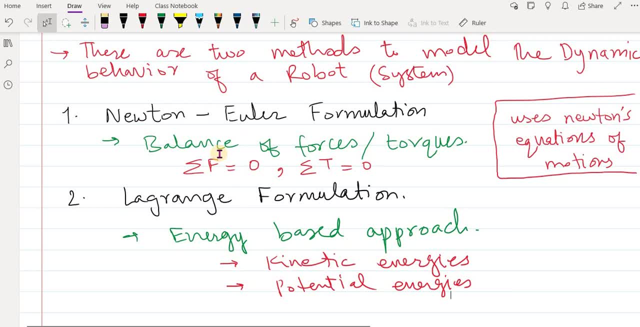 We shall briefly have A very Simple example For both, But eventually we shall stick to the Lagrange formulation, Because this is A. This is more Advanced approach, This is more Systematic approach And, Yeah, I personally Prefer this approach As compared to Newton approach. So whenever we Model our robot, 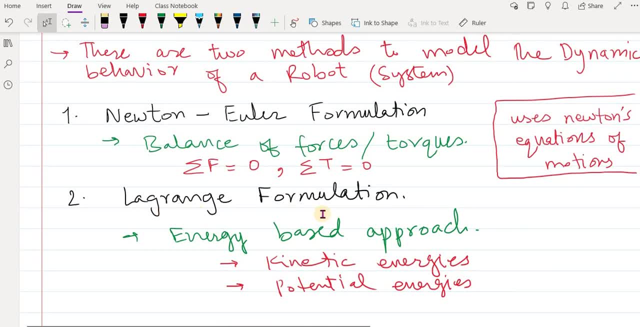 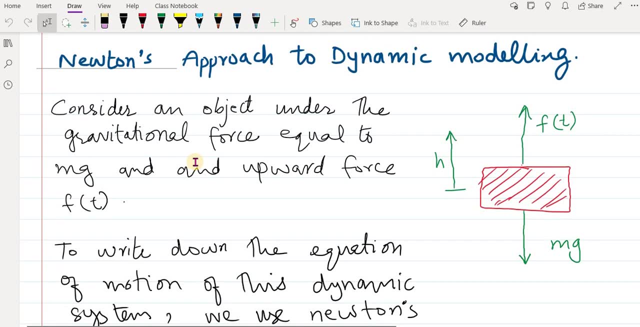 We shall prefer modeling with Lagrange formulation. But we also should Know about the Newton approach. So let's see how Newton approach to dynamic modeling Works. So let us Consider an object under the Gravitational force equal to Mg. so here you see that We have an object here. 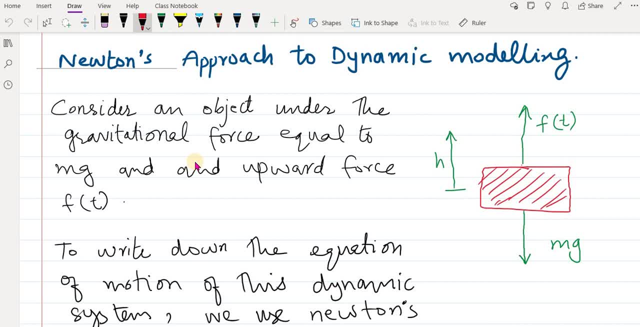 This red color object, And it is Um, Two forces Are acting on it. One is the gravitational force, And then there is a force That is applied To this object And it is acting upward, Opposite to your Gravitational force, And the And the movement. The motion is along. 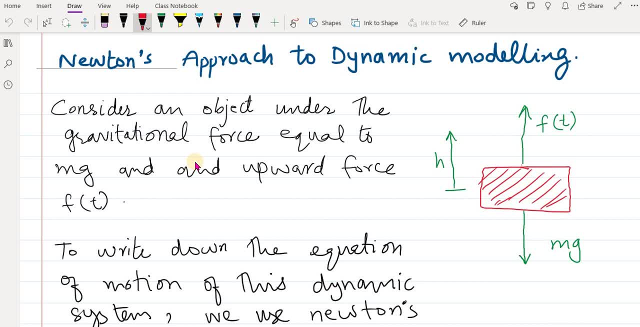 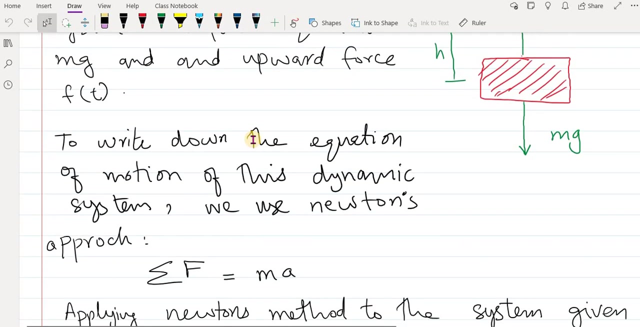 The- You can say Y axis And H is the Coordinate. you can say H is the generalized coordinate. That is happening. Okay, To write down the equation of motion For this dynamic system, We Use Newton's approach. So Usually what the In the Newton approach, As we already discussed, 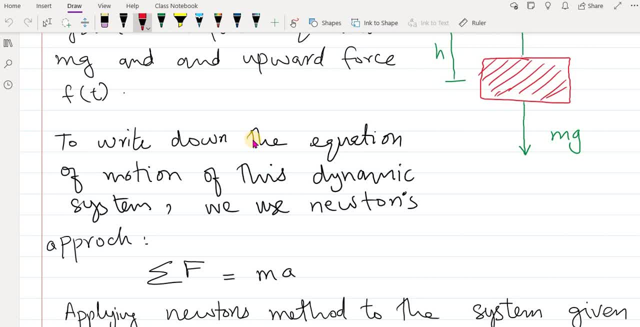 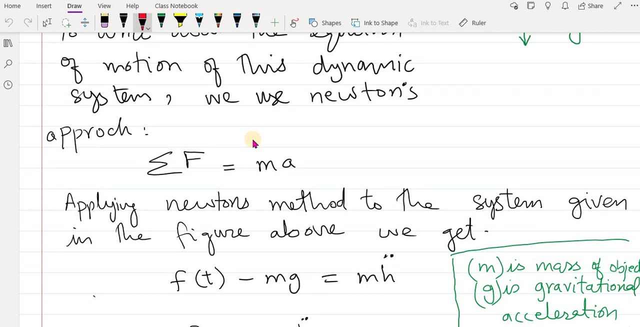 We use Newton's equation of motions And where it says That sum of all the forces Is equal to, Uh, Mass into acceleration, And So this is not Sum, This is Force is equal to Mass into acceleration. And then we can use Sum of all the forces Is equal to. 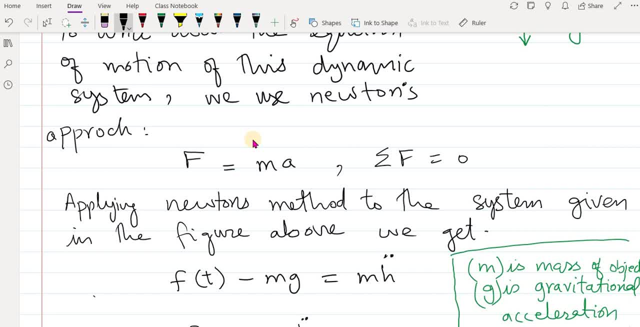 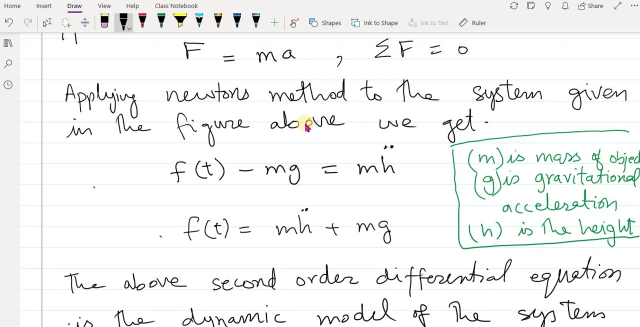 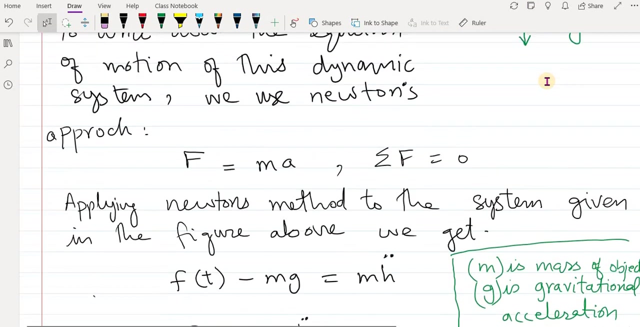 Zero, Or This can be also Translated to that Force is equal to Force dissipated. So applying Newton's method To the system given in the figure above We get. So Here we apply when the Newton's method. We see that this is our applied force And This is the downward force. 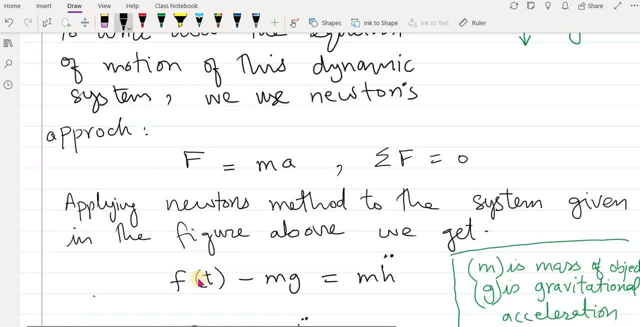 Which is acting downward. So applied force, Uh Minus the, The downward force is equal to: Uh, M, H, double dot. Okay, we are using this equation Here, Um, This equation, So it says that The forces, that is, Uh, That are acting On the robot, On this object, Their sum is equal to: 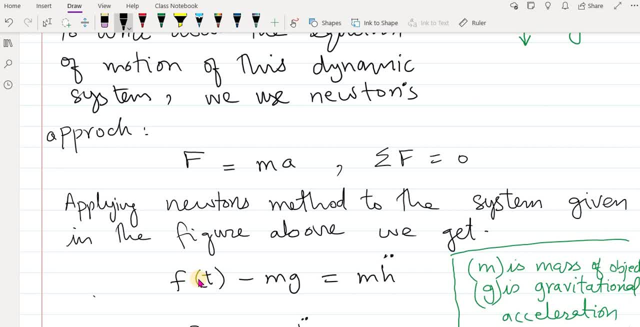 Mass into Acceleration. So So actually these both. So here we can. it means it's okay to write the sum, Yeah, so I think we can write here The sum And we can write Here also. So this is also, if We take this term in this here, Then sum of all the forces. 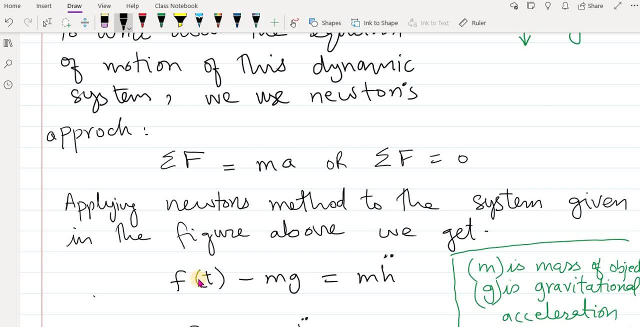 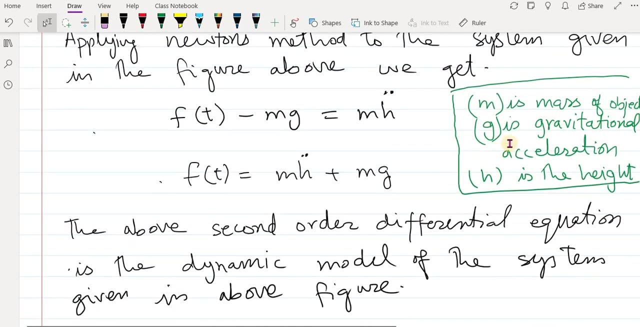 Will become zero. yeah, So, Using this equation above, So it means that Some of these two forces Will result in this motion, Which is M- H double dot, Where M Is the mass of an object, G is the gravitational acceleration And H is the height. The above second order differential equation. 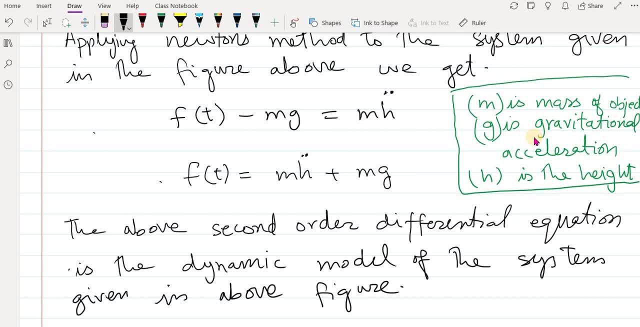 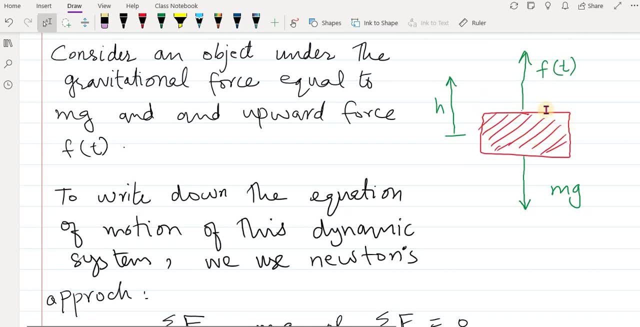 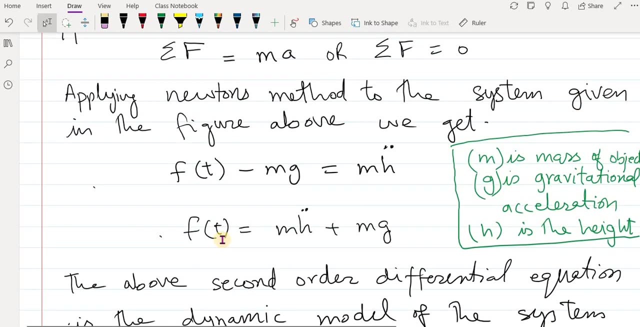 Is the dynamic model of the systems, Of the system Given in the above figure. So it means that This, To write the dynamic model Of this system, This object- We can use this equation here. Okay, And this equation says that Applied force is equal to The motion About uh. 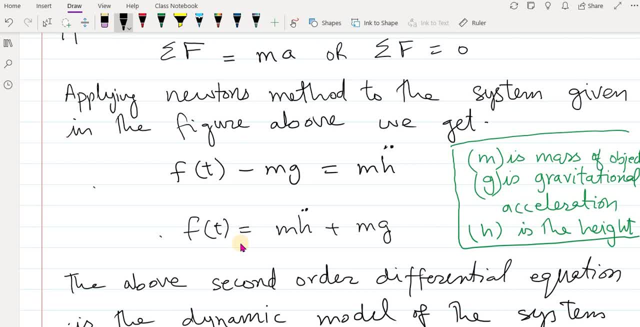 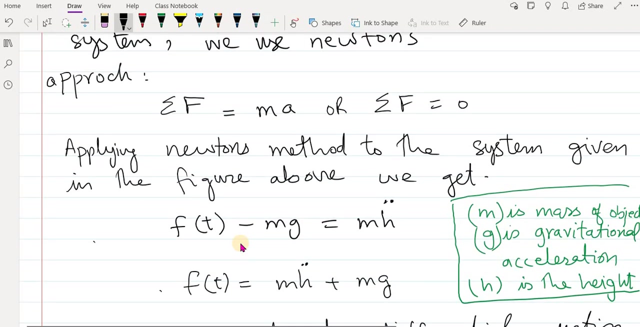 Your generalized Coordinate H Plus The gravitational force. So it means that whatever force You apply on the object, It will be translated To the motion of the Of your object plus The work done against the gravity. Okay, So this is Um, This is the dynamic model Of the system. 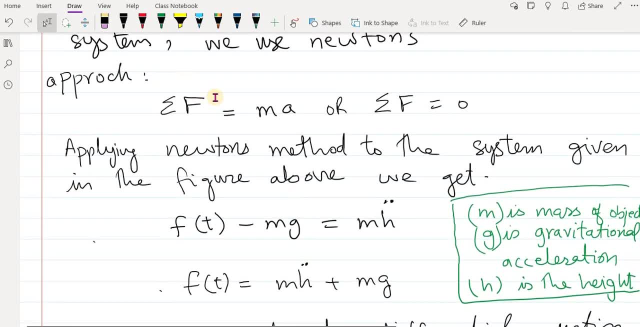 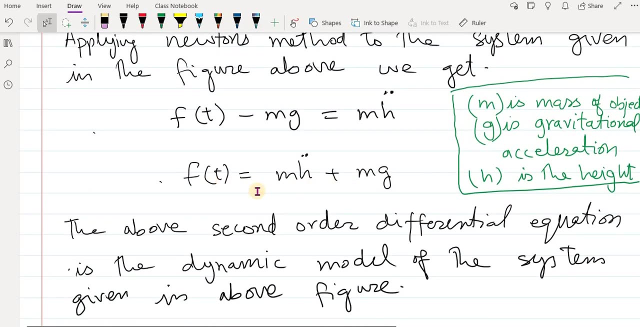 It's that simple. Just use the Newton equation of motion And Just say that sum of all the forces Is equal to either Zero or mass- into acceleration And then put the Values of the forces- And remember that These are not always forces, They can also be torques. 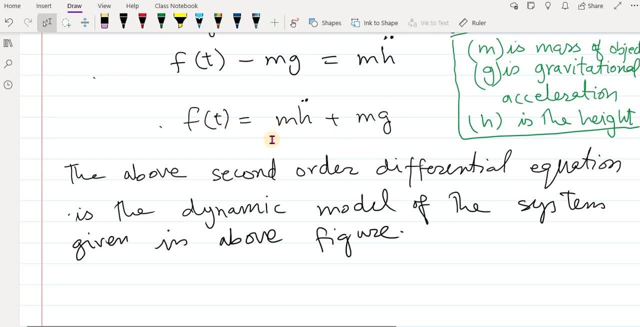 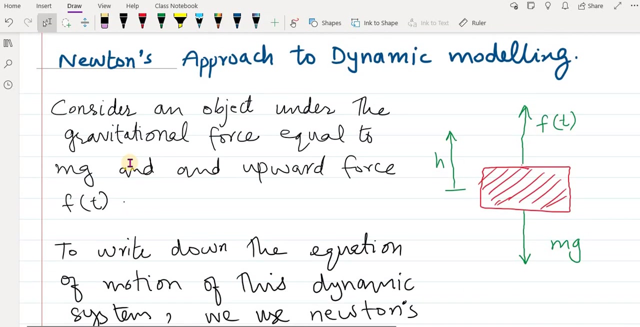 So this is the Dynamic model, And remember that we said that In the Dynamic model there is always forces And motions involved. So here you have motion And you can calculate the force, Or you have a force, you can calculate The motion. So this was one method To model a dynamic system. 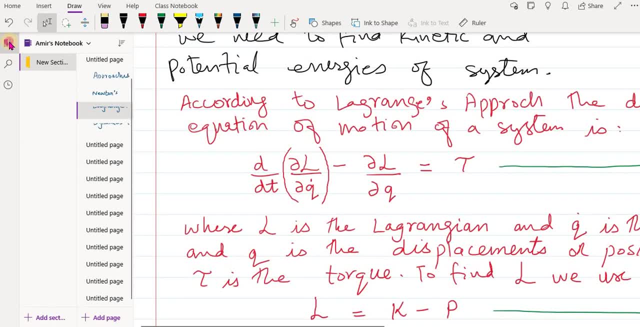 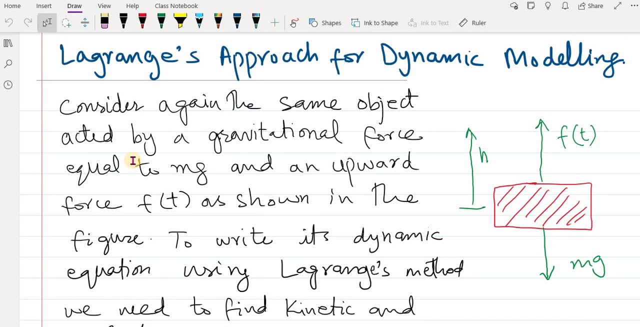 Now let's see another method To calculate the dynamic System. And this second method, we already Know that It's called Lagrange's approach For dynamic modeling. Consider again the same object Acted by A gravitational force Equal to mg And an upward force F of t, As shown in the figure. 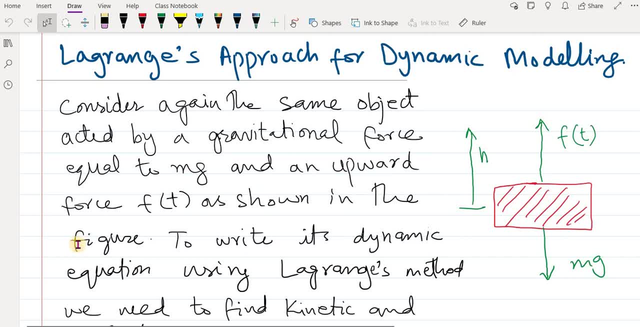 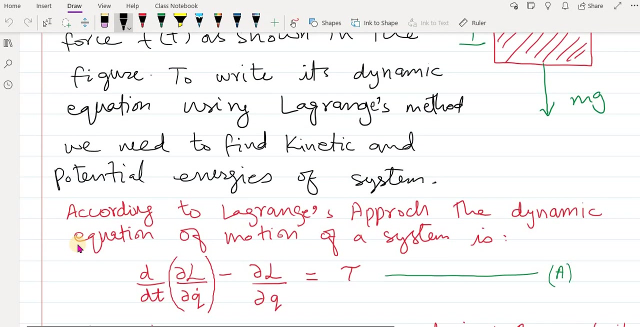 So this time again We have same object And it is Applied force is F of t And the downward force is Gravitational force, mg, And the generalized coordinate of motion Is h. To write its Dynamic equation Using Lagrange's Method, we need to Find kinetic and potential energies. 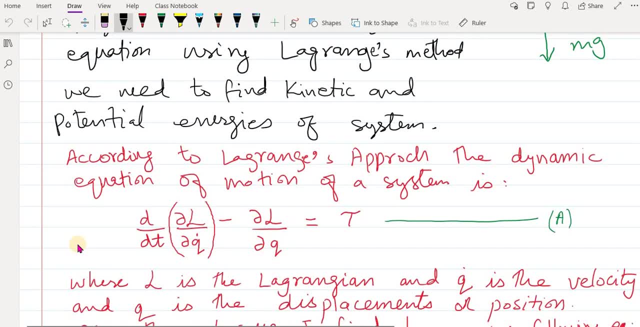 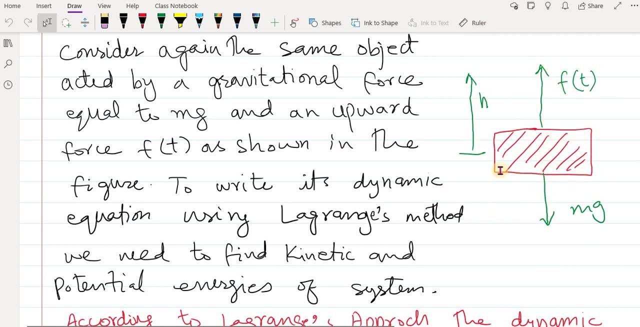 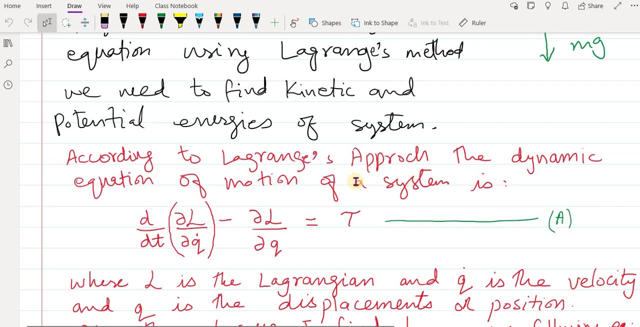 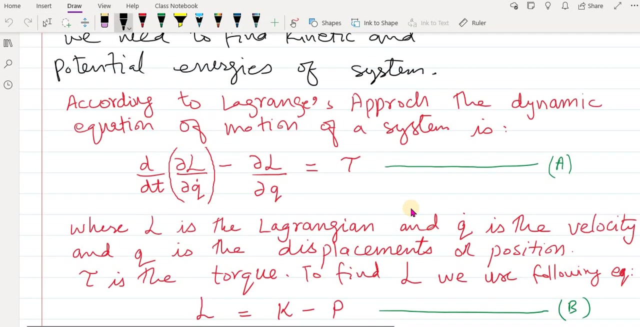 Of system. So Now we want to write The dynamic equation Of this Motion of this object Or this system. So what's a Lagrange's approach says? According to Lagrange's approach, The dynamic equation of the motion Of a system is: It can be written as this: 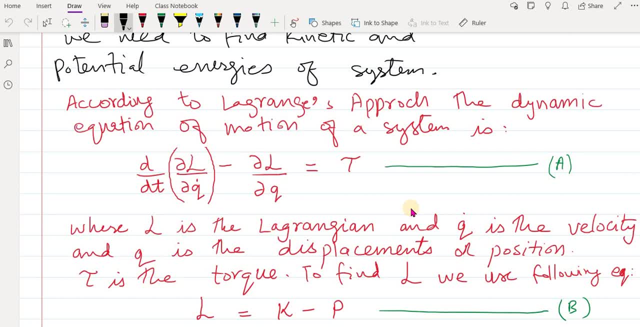 This equation, This is the equation of motion Using Lagrange's approach. So what? This equation of Motion says that This is a time derivative: d over dt, This is a time derivative And this partial derivative, Partial Lagrange, Lagrangian, Is a symbol for A special symbol. 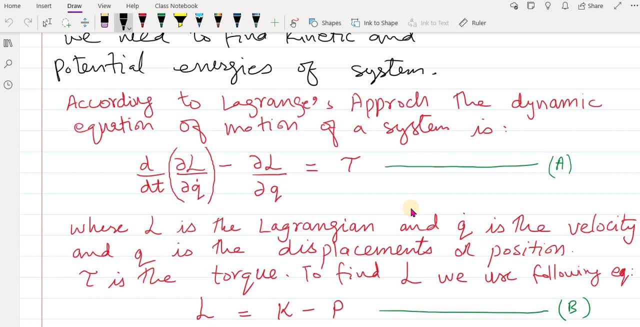 For Lagrangian, And later we see that What's this Lagrangian? l, And then Partial derivative With respect to velocity. This q is the Motion Coordinate, Motion Variable. you can say: And this dot means Derivative of this. If it's a linear motion It will be x dot. 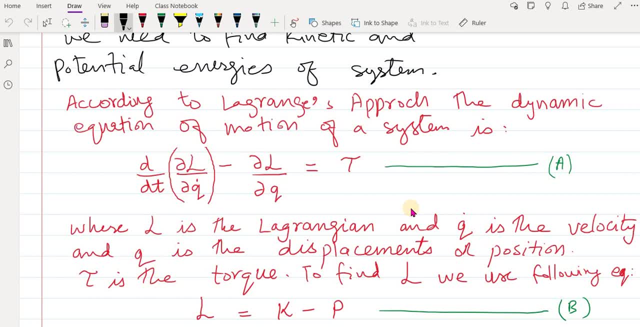 Which is a linear velocity. If it's a angular motion, Then it will be theta Dot, which is an angular velocity. Then we have minus, Then partial derivative of Lagrangian Over partial derivative Of your Motion. variable: Either theta Or it can also be x Or y or z, whatever. 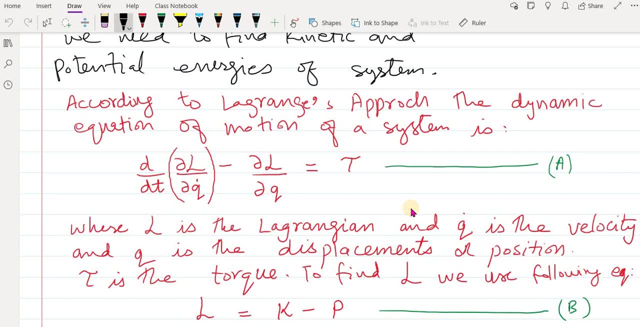 This is equal to Tau. Tau is the applied force, or Torque depends upon What's your System is, What is the input to your system is. So we name this equation a, And This equation is a generalized Equation of motion according to Lagrangian's approach. So where? 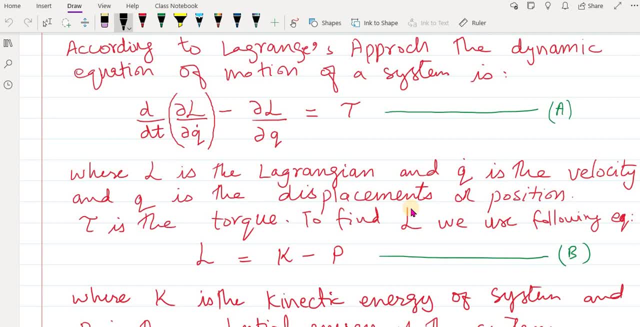 Lagrangian is the Lagrangian And q dot is the velocity And q is the displacement Or position Which we say q is a motion Variable, Tau is the torque, Or it can also be force. To find Lagrangian We use following equation: So what is Lagrangian? 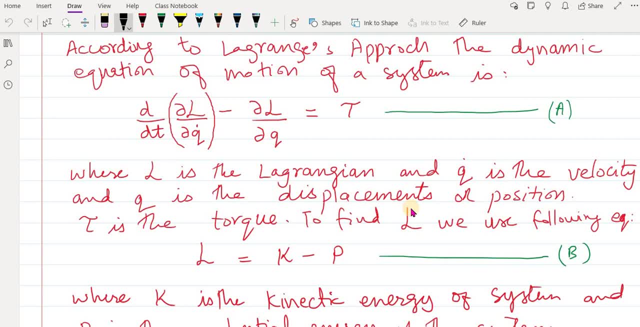 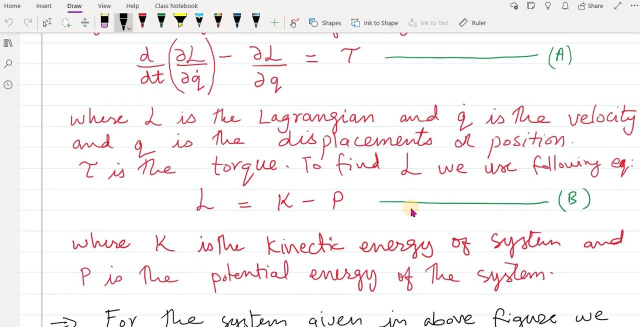 Lagrangian is just: a Is a difference between the Kinetic and potential energy Of a system. This is a case of The kinetic energy of a system And p is the potential energy of a system. And then you take a difference And you get the Lagrangian. 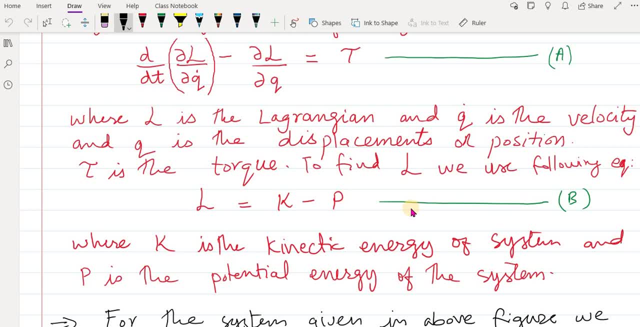 And Then you Put this Lagrangian here In the equation a, And then you take Its partial derivative with respect to velocity And then take the Derivative again with respect to time And then subtract this term From the partial derivative of Lagrangian which comes from here. 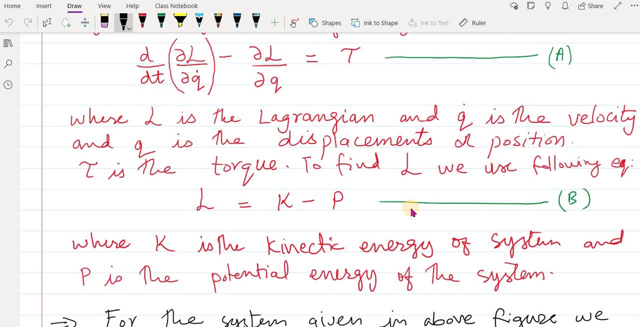 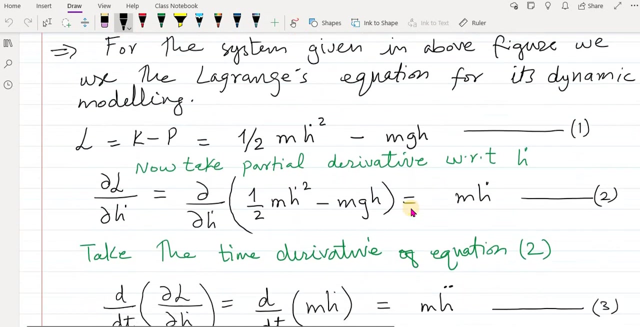 And take its partial derivative With respect to position And then subtract these two terms To get the, The Value which is equal to your applied Force or torque. So this is the second method To model the dynamic equation Dynamic system. For the system given in the above figure, We use the Lagrangian's. 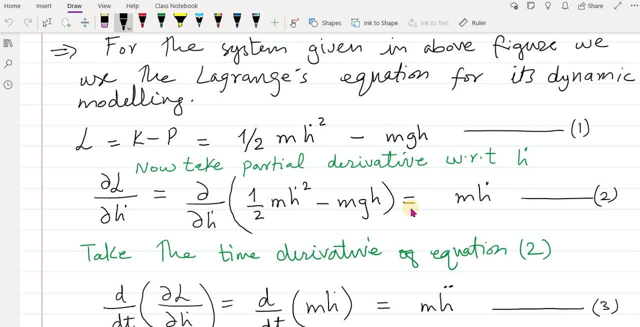 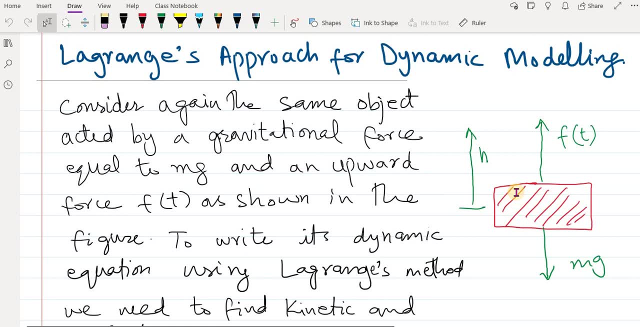 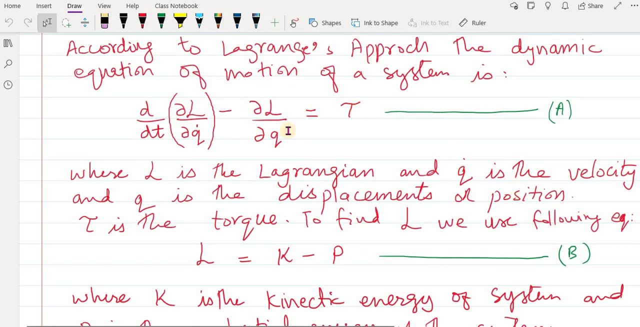 Equation, for Its dynamic modeling. So for Our system That we have described here, Now let's try to model this system With respect to Using the Lagrangian's approach. So what Lagrangian's approach? Say that first you Need to calculate the, The kinetic energy And potential energy. 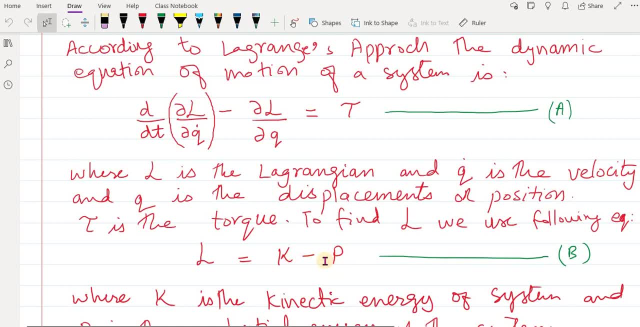 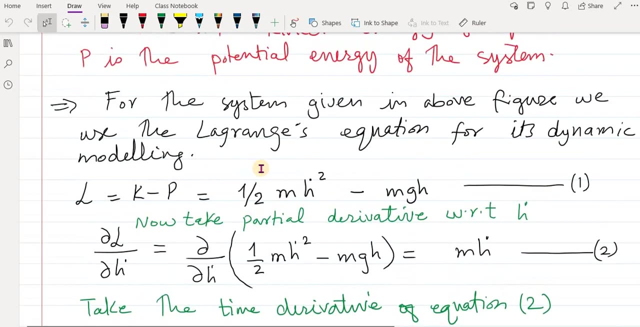 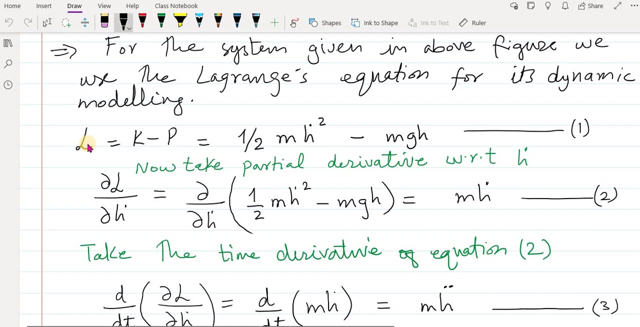 And then, once you have The kinetic and potential energies, Then you Take a difference and get the Lagrangian And then Use this equation to find The equation of motion. So So That's what we are doing here. We have here the First of all. we need the 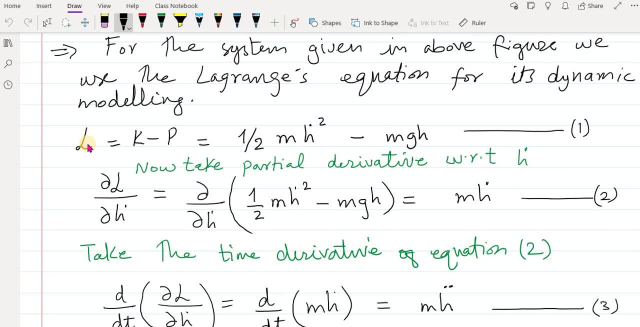 Lagrangian, And which is the, Which is the difference between the kinetic And potential energy And the kinetic energy of the system. You know that kinetic energy is Half mv square. Okay, We can write here: K is equal to Half mv Square and P is equal to mgh. 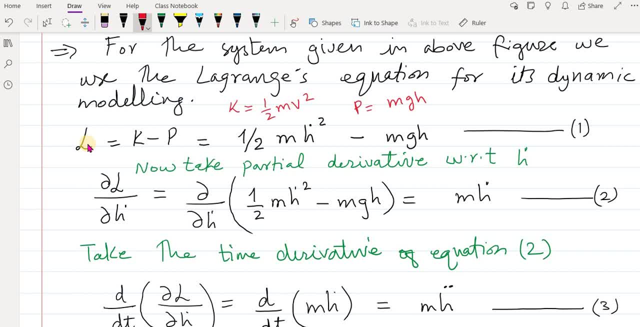 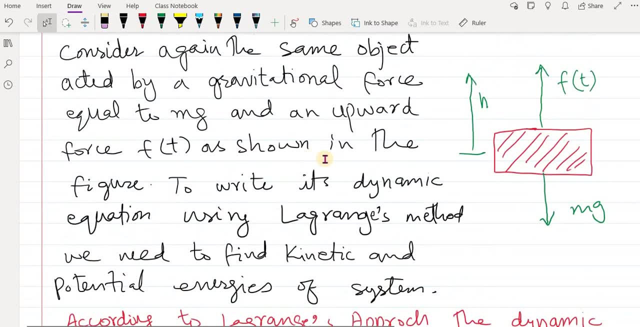 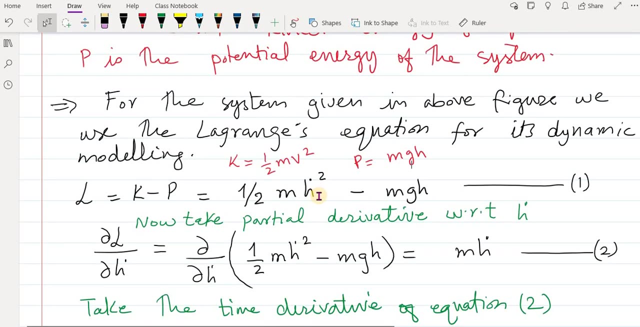 So, putting The values here, We have Velocity Along this X axis, which is our H. so if we take a Derivative of H, We get the velocity Okay, because Velocity is the derivative of Displacement time derivative. So that's What we have represented here: Half mh dot square. 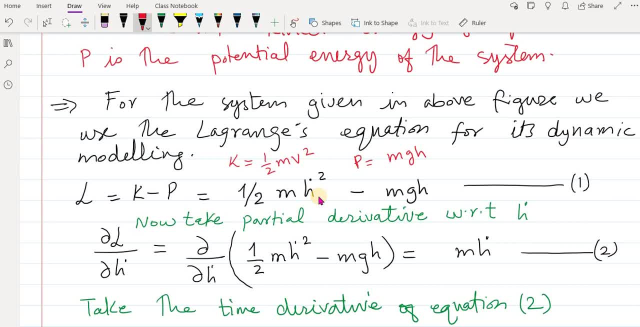 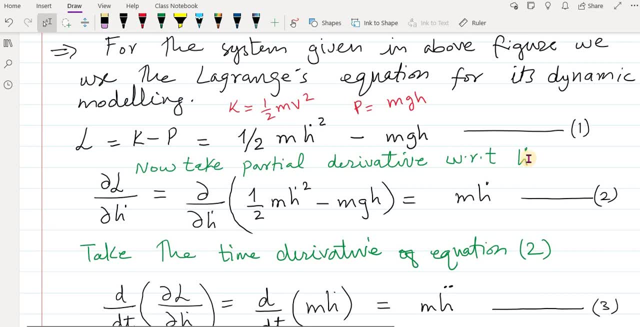 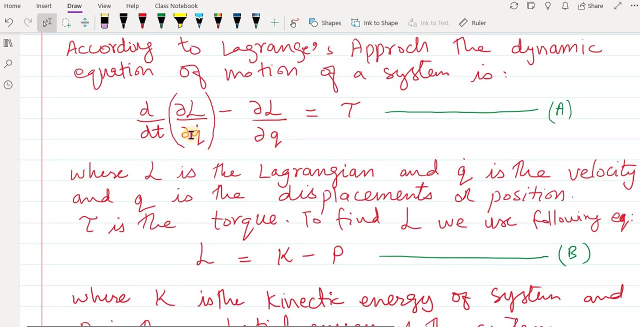 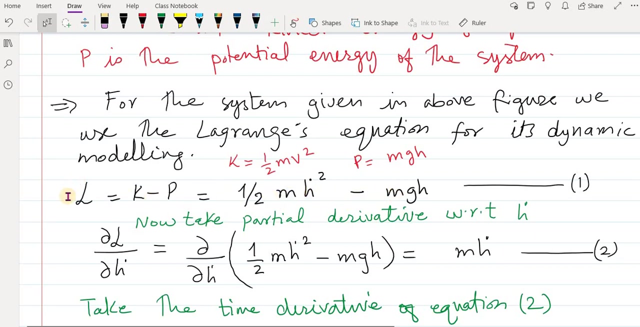 And then minus The potential energy, Which is mgh. So Now take partial derivative With respect to H dot. So, Because we have to use this equation A, We have already calculated Lagrangian, Because we have calculated The difference of the kinetic and potential energy, And which is Lagrangian. 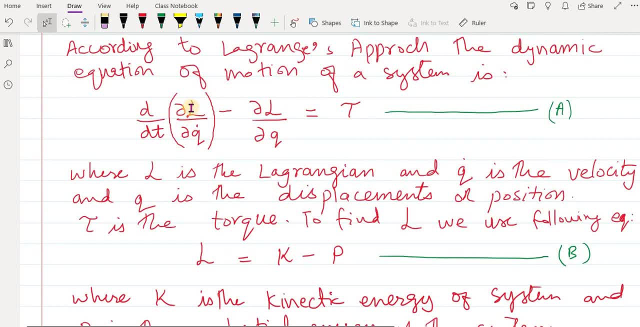 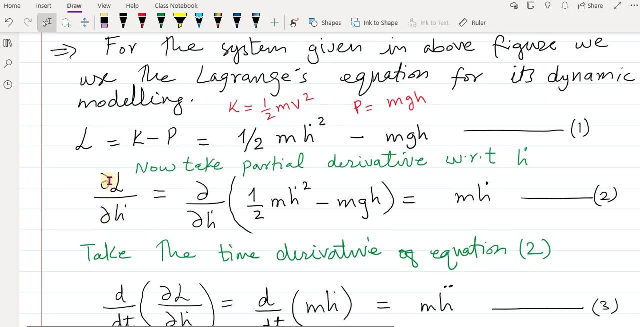 Now we have to put this Lagrangian Here, And then we have to take the partial derivative With respect to velocity. So that's what we are doing here: We are taking here the partial derivative Of Lagrangian with respect to the velocity, Which is H dot. 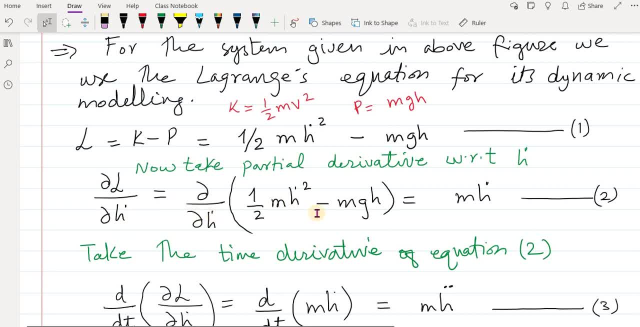 And this is equal to Lagrangian, is equal to The difference of kinetic and Potential energy. If you take the derivative, Then This term, here It will be: This is a constant, 1 by 2, And m is a constant. It will remain like this. And H dot. 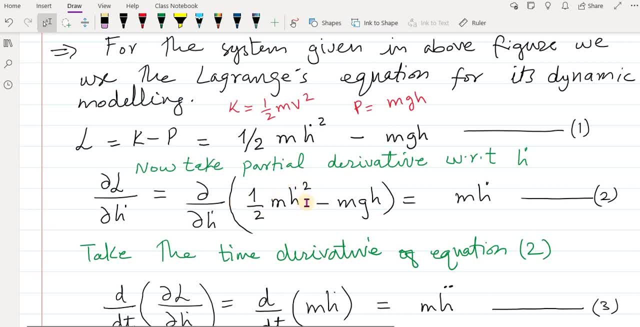 It will be: 2 will be multiplied here, And 2 minus 1 Is 1 And this derivative will be: And this 2, And this 2 will get cancelled, So it will be mh dot. So, Which means mass into velocity Minus, This term becomes 0. 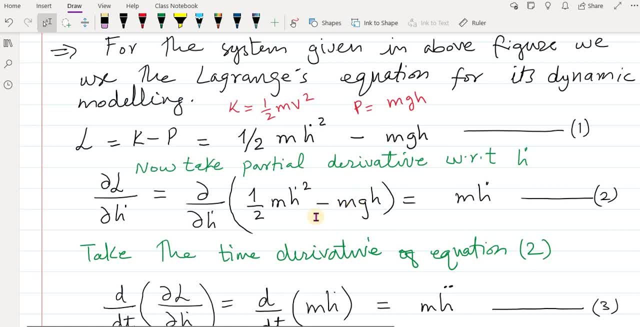 Because this is Because here, With respect to Velocity, This is a constant. If we take a partial derivative, with respect to velocity, This is a constant. If you take a derivative of constant, It will be 0. So your final answer will be mh dot, Which means that mass into velocity. 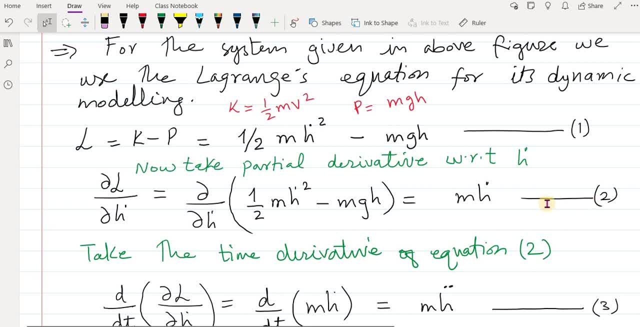 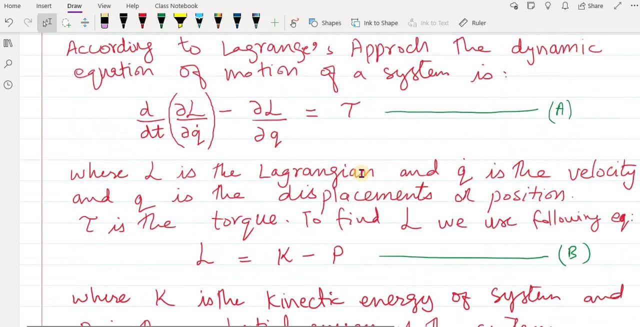 We name this equation As equation 2. Now take the time Derivative of equation 2. Why we are doing it? Because, again, according to Lagrangian, Lagrangian's approach, We have to first take the partial derivative, Which we have already done. Now we have to take the time derivative here. 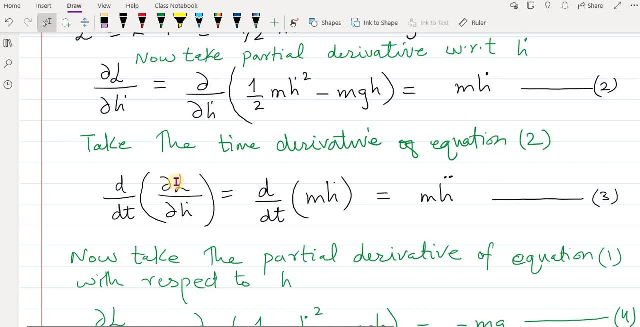 That's what we are doing here. We are taking the time derivative of Our Equation 2, Which says that d over dt of the Partial derivative of Lagrangian Over partial derivative Of with respect to Velocity, And this is equal to d by dt over Of mh dot. 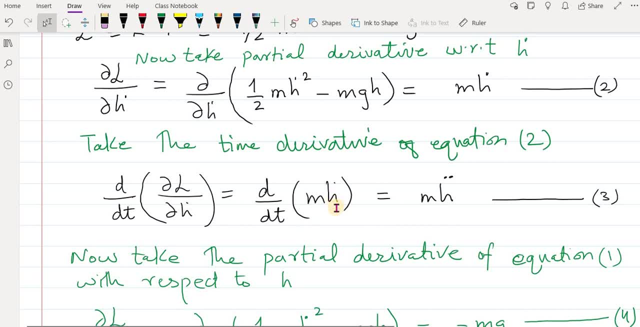 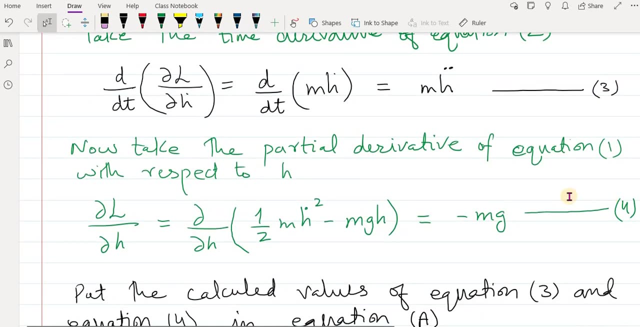 So if you take a time derivative of mh dot, It will be mh double dot. Because the derivative of Velocity Is acceleration and m is Constant, We name this equation as equation 3. Now take the partial derivative Of equation 1 With respect to h. So For Lagrangian's, 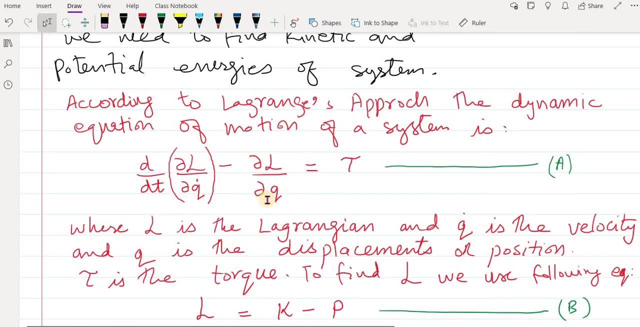 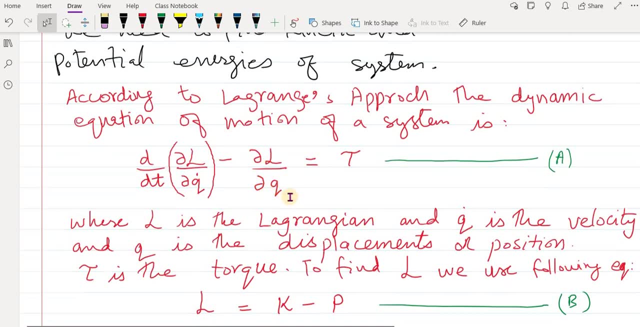 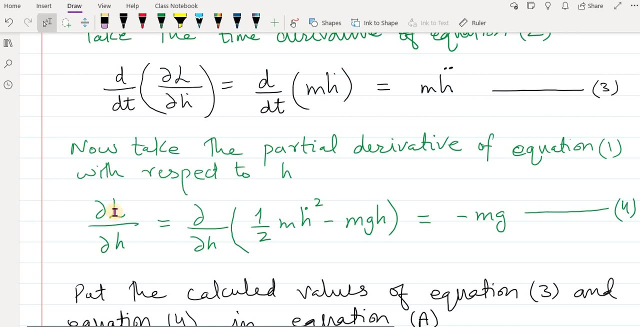 Approach. We also need this term here, Where we are taking partial derivative Of Lagrangian With respect to position. So That's what we are doing here: We are Taking partial derivative of Lagrangian With respect to the Position, and If you do that, Partial derivative Of this term will be 0. 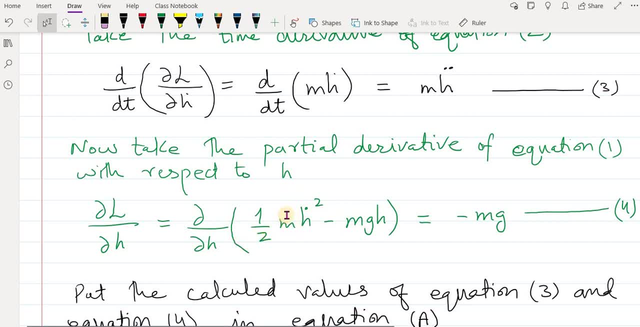 Because Here we don't have any position variable. All of them are Constant. So This velocity is actually a variable, But since We are only taking partial derivative With respect to the Position, so in this case This will also be treated as constant And all term will become 0. 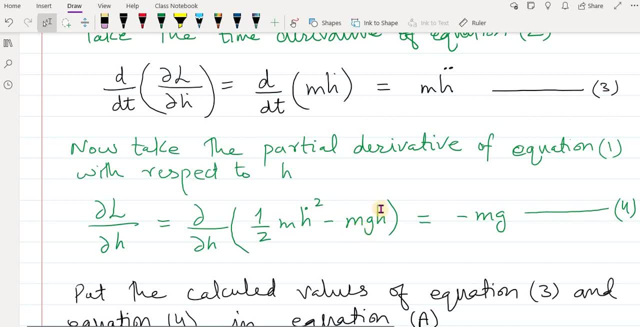 And then we have a second term Where we have a variable h, The position, And if you take another, two Are the constants, And if you take the partial derivative Of this term, it will be Minus mg. So the answer will be Minus mg and this We name this equation as equation 4. 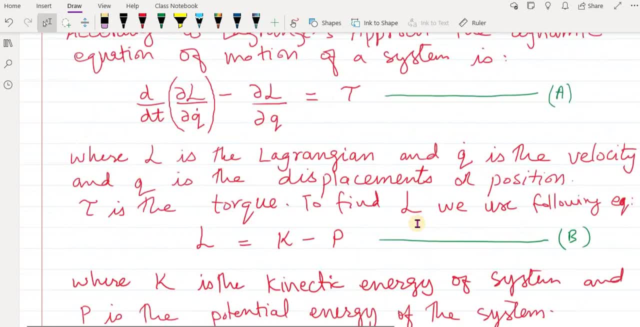 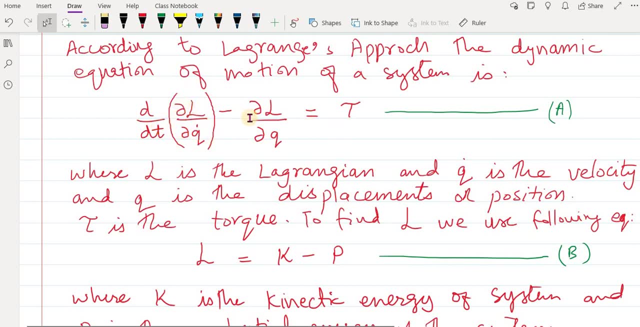 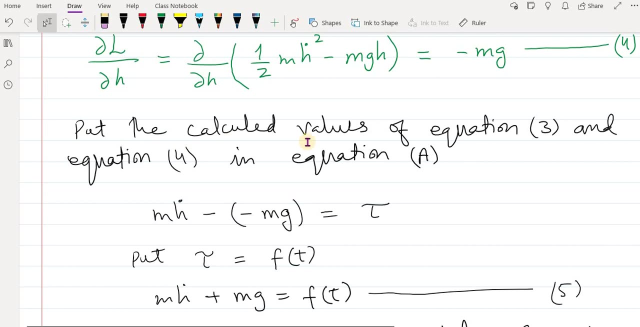 Now we have calculated all the terms Related to the Equation of motion According to the Lagrangian's approach, Put the values of this Term and this term and also Here this term, So Put the calculated Values of equation 3 and equation 4 In the equation a. 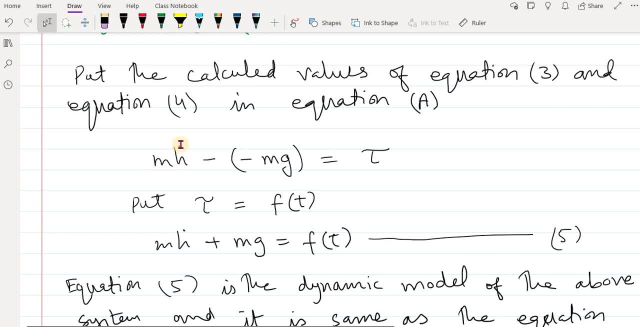 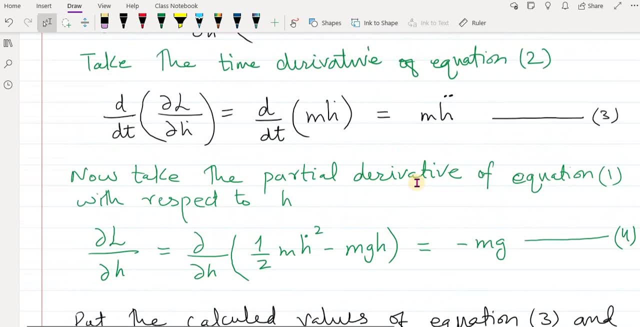 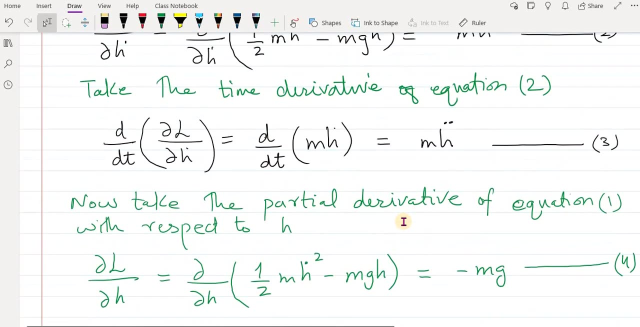 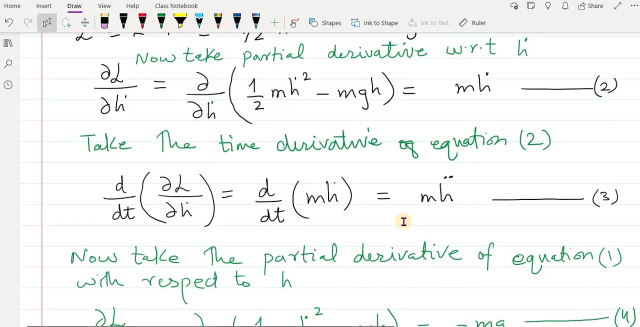 What we get here: m h dot Minus mg, Which comes from here, And m h dot Comes from here. And And Is it dot or is it double dot? Yes, It's double dot. It's not m h dot, It's m h double dot. So let me correct it here. 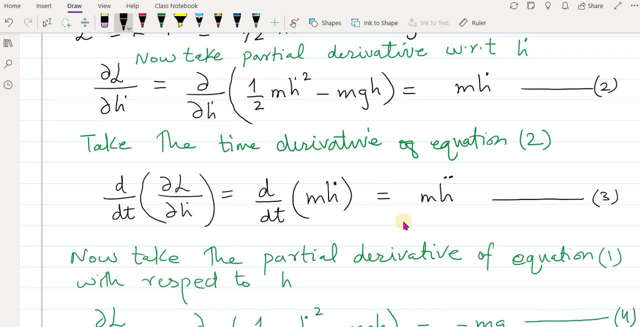 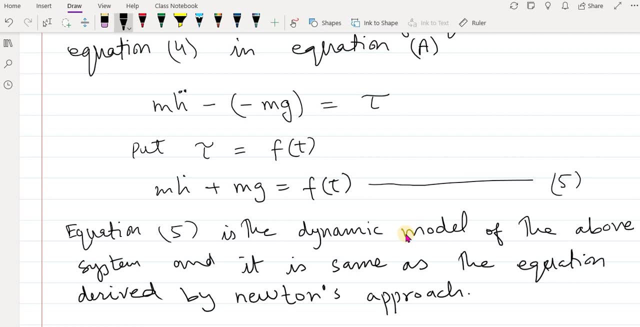 So this is single Dot here and The answer is double dot. So here the answer will be m, h, double dot And minus minus mg is equal to Applied force Or applied torque. So in this our case, we have The applied torque, is actually applied force Which is acting upward. 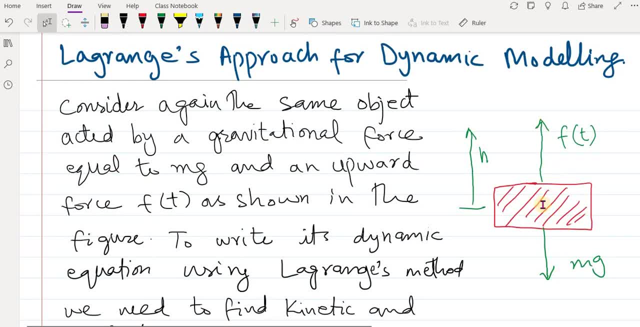 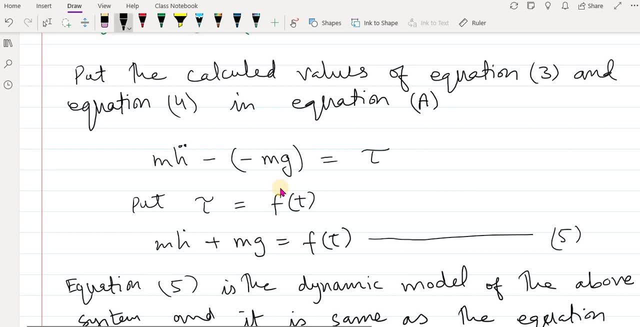 In this figure. This is the applied force Upward. so we put the Value of tau is equal to F of t and we put it in the Equation here and we get This nice dynamic Equation of motion which says that The If you apply a force F of t on an object, 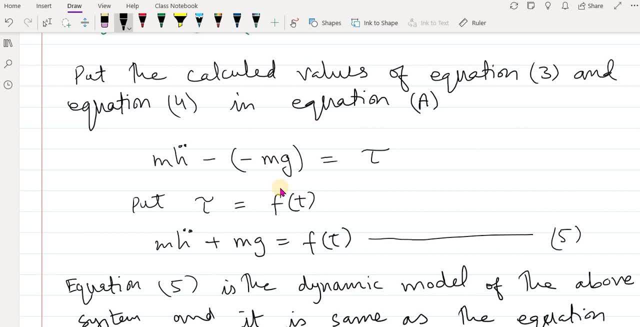 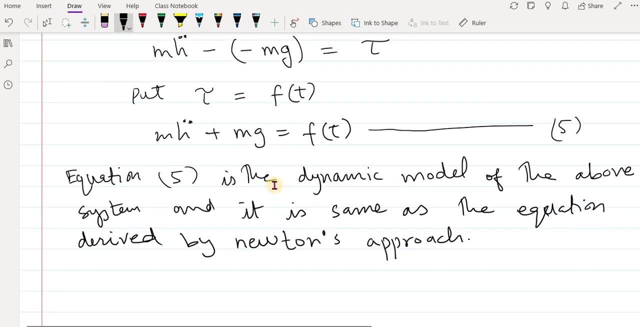 Under gravity. This force will be Compensated by The gravitational force Which is acting downward And also this force will result In the motion equal to m h double dot. We name this equation 5, Which is the dynamic model of the System. Equation 5 is the dynamic model of the. 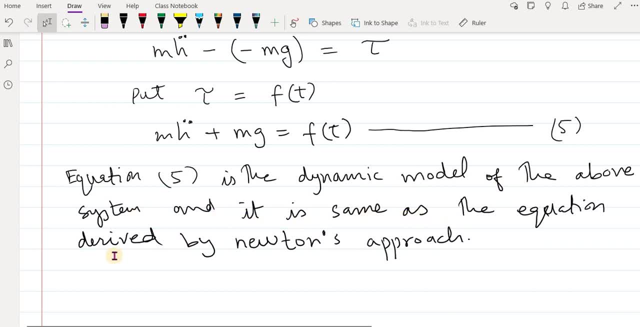 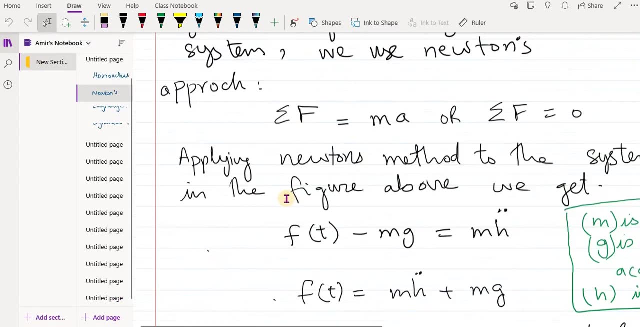 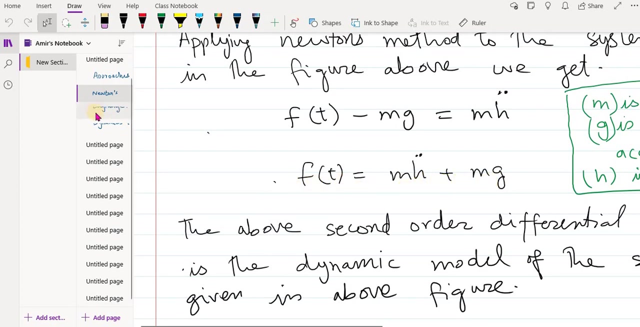 Above system and it is Same as the equation derived By Newton's approach. So If you remember that, The Newton approach, What was the dynamic model there? So this was here: m, h, double dot plus mg is equal to Ft. so Here we have same. So you see that. 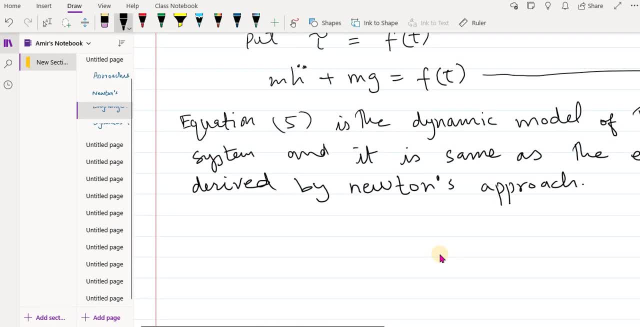 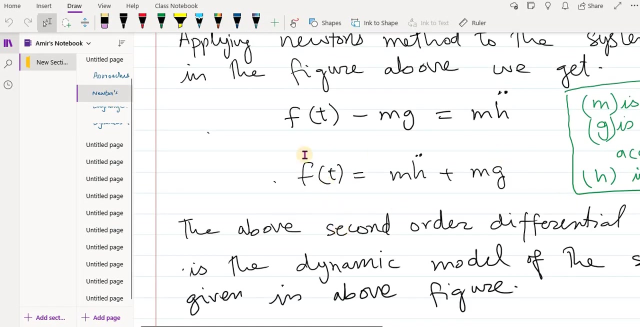 Or you can rewrite it To look like Same: M, h, double dot plus mg. So you see that It doesn't matter if you model the system Using Lagrangian Lagrangian method or Newton method. The equation of motion, Dynamic equation of motion, Will be same. So in this simple 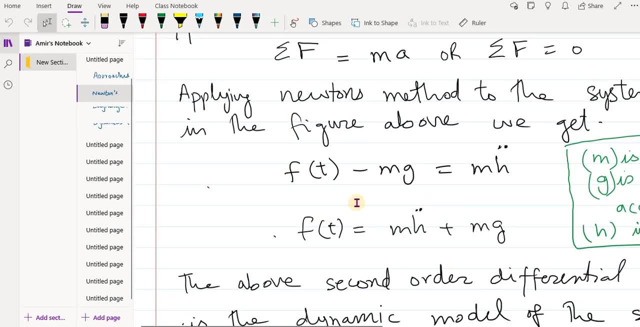 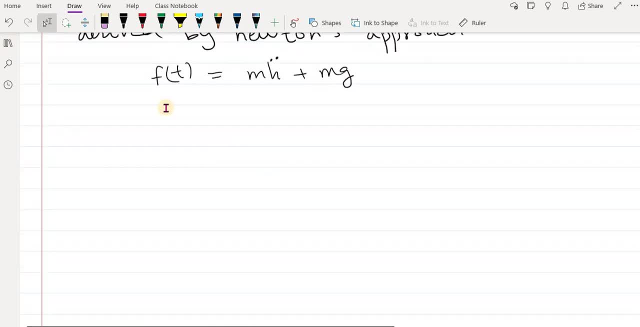 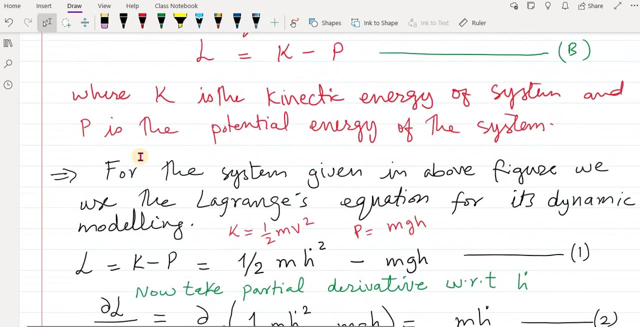 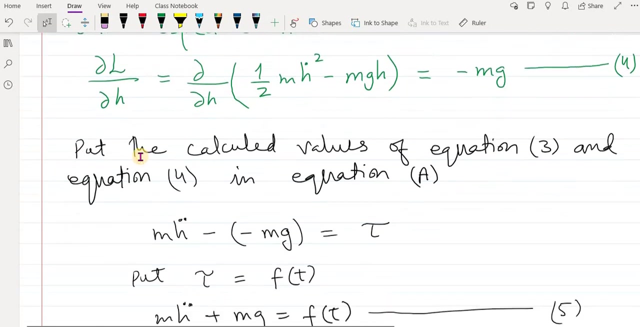 Example. you see that Newton approach looks Very easier, only Just one or two steps. But here Lagrange's approach, It looks a little bit Difficult, But for Complex systems This is other way Around. If your system is complex There are lot of variables involved, Lot of forces, lot of torques. 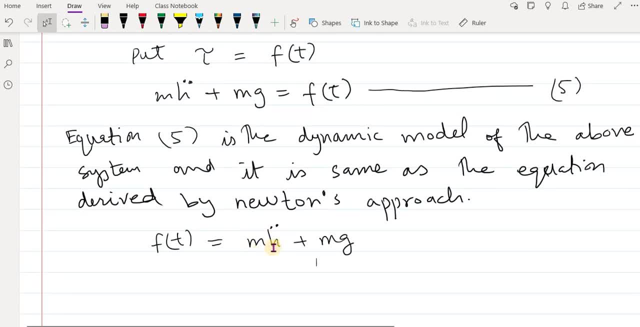 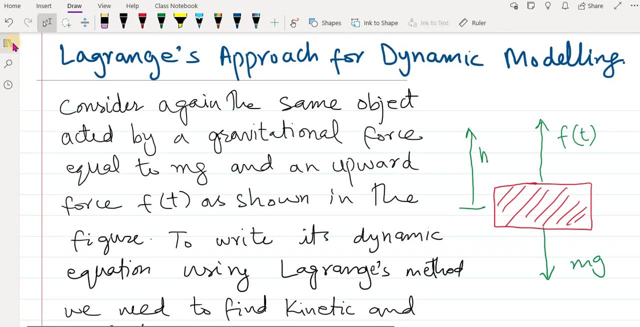 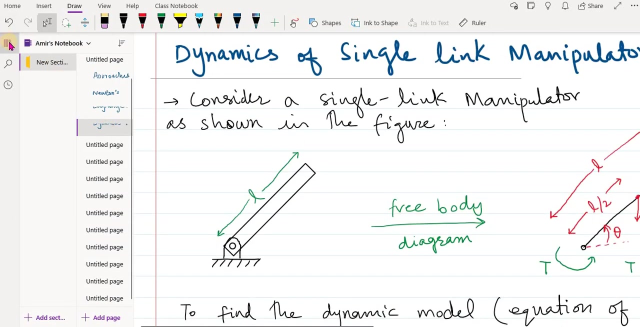 Then this method becomes Actually easier to Model your system. So that's why we stick with this Approach. So we have seen A very simple basic example How to model a Dynamic system. And for In case of robotics, Let's see how we can model Our robot using Lagrange's approach. 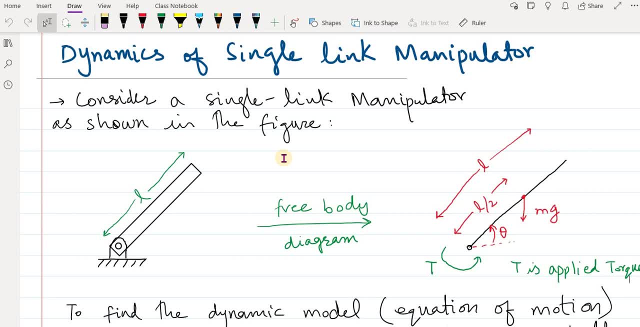 How we can Get the dynamic model of The system. So let's take an example And consider a single link Manipulator as shown in the figure. So we have here a Single link robotic Manipulator And We have here a fixed joint, And then there is a link. 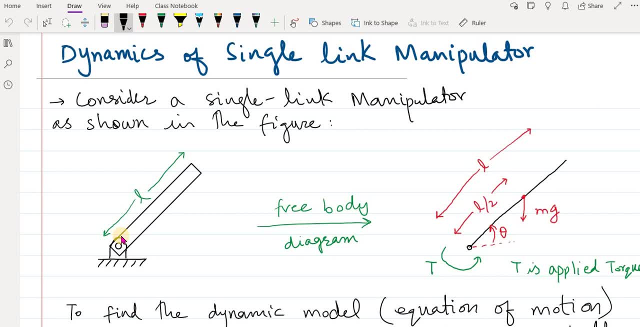 Here, and the length Of this link is L- And, Apparently, if there is some Kind of torque acting on this Torque acting on this robot, This torque is coming from The motor, let's say The motor that's attached with this Robot, and So The first step we do is we draw the free body. 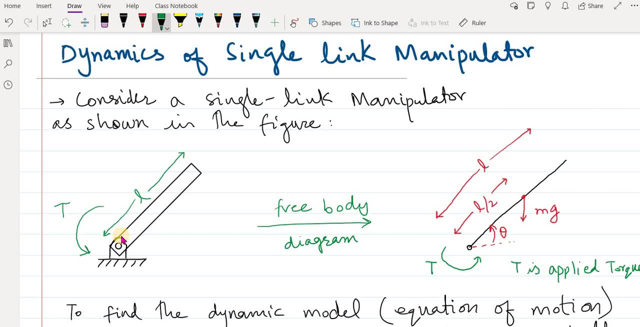 Diagram Because It's easier to work with. So we have drawn the Free body diagram. this is a link. Black color line: this is a joint And the torque T is Applied. torque On this link, robotic arm Link And the center of the mass Here. this is the center. 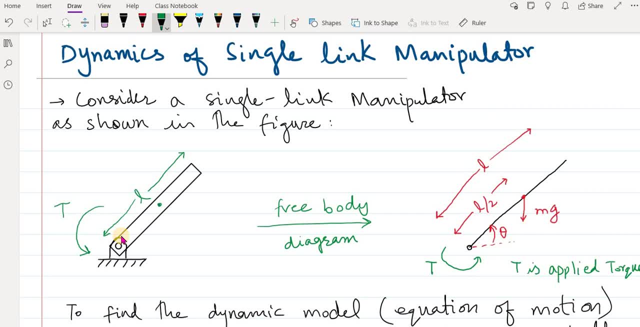 Of the mass. So The gravitational force, We always Consider that it's acting on the center of Your whole mass. Okay, and So that's why we say that The force acting downward, mg, Is acting on the center of this Link, and The length of the Center is L by 2. 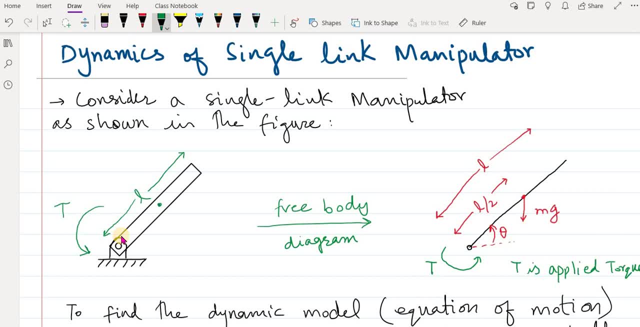 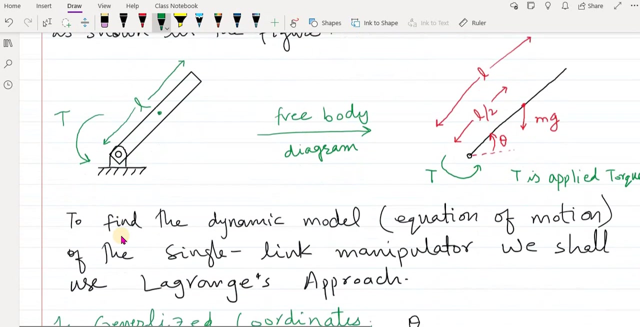 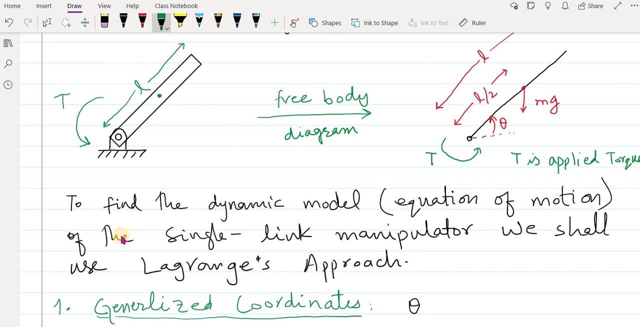 The Motion Coordinate of this robot is actually This theta. so This link is rotating About About an Axis, let's say z-axis, And the The motion Variable is theta. So now we have a free body Diagram to find The dynamic model or The equation of motion of A single link. manipulator. 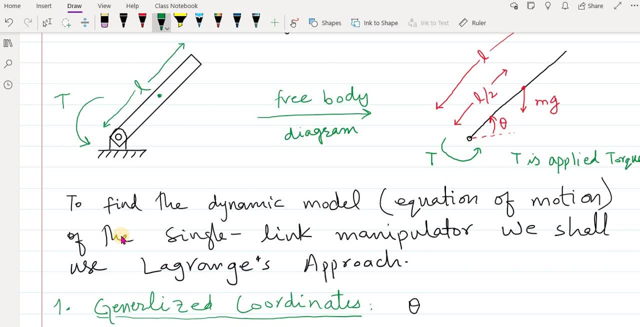 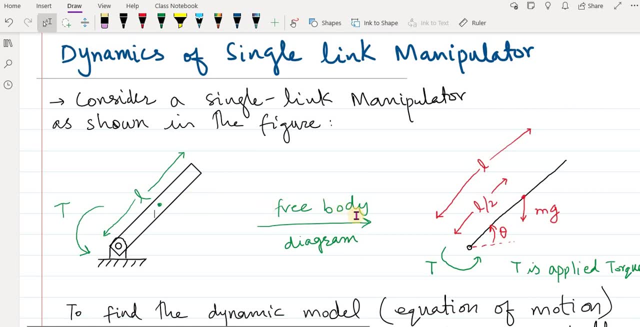 We shall use Lagrange's approach. So what we are interested in? we are Interested in finding a dynamic Equation or a dynamic model Of this robot Which can relate the Applied torque to The motions, To the acceleration velocity And position of this Robotic arm. So, Again, we just follow the steps. 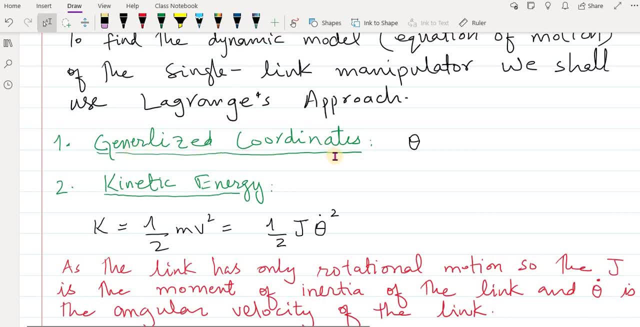 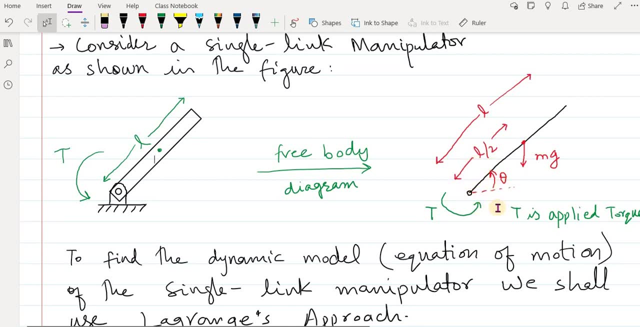 So first you need to identify what are the Generalized coordinates here, Or where, along Which coordinates, which axis The motion is happening. Okay, for in this case The motion is, Or is the rotation about Z-axis, let's say, and the Motion variable is theta. So you need to. 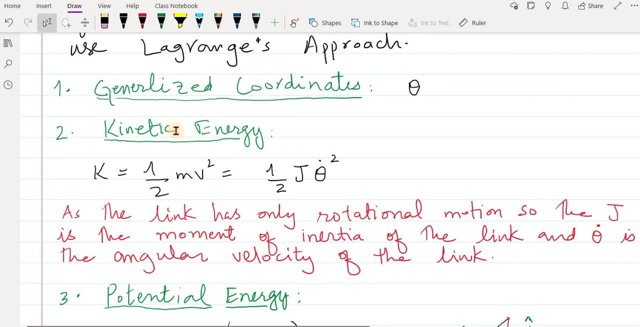 Identify this variable, theta. Once you have done it, The second step is you have to find the Kinetic energy. Why we are doing it? because We need to Put values Of the Of the Kinetic energy, Potential energy, to find the Lagrangian. and then we have to. 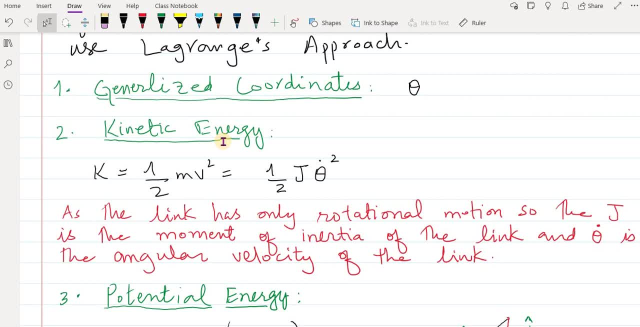 Also put the values of Lagrangian and take its Derivative and partial derivative To solve the, The equation of Motion, using the Lagrange's Approach, So how we can Calculate the kinetic energy. We know that kinetic energy is equal to half mv square and In our case, because we have 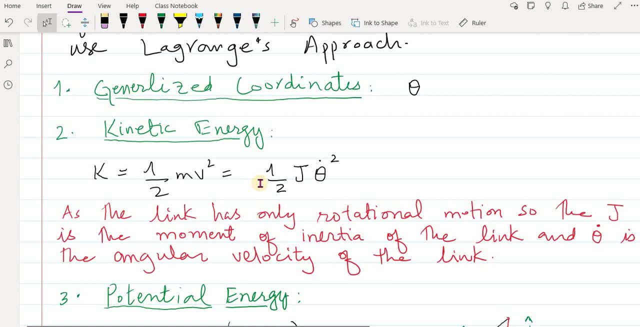 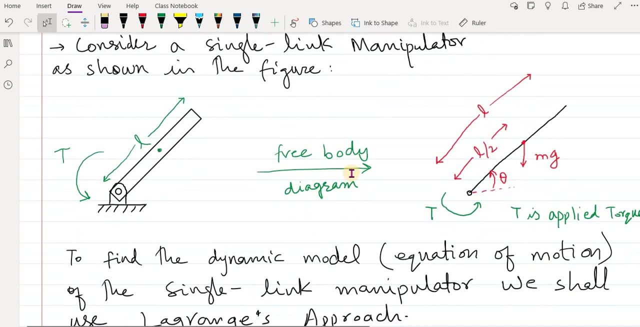 A rotation. Okay, so We can write it as 1 by 2, j, theta Dot square. What is the j? J is the. This is we have: Center of mass is c And j is the. J is the moment of Inertia, because You remember when the mass is. 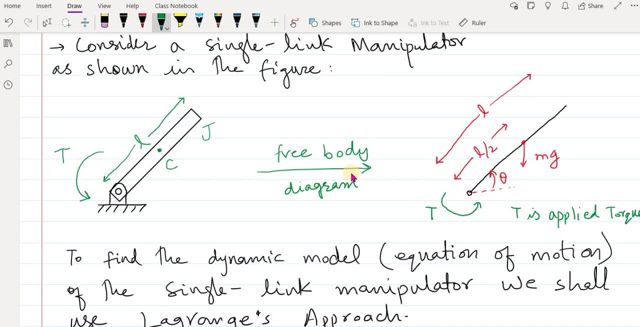 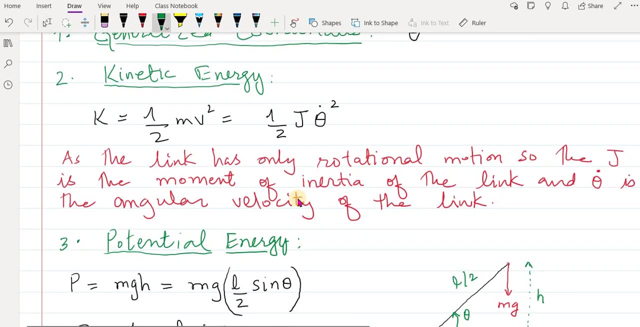 Rotating. okay, So we use J, which is the moment of inertia. In this case there is A rotation, so we shall use J instead of m, and we shall Use theta instead of X or y, As a Link has only rotational motion, So the j is The moment of inertia of the link. 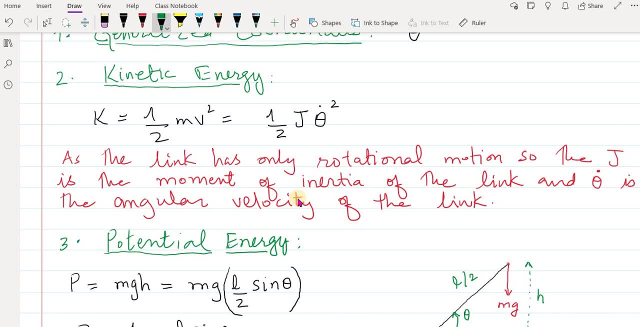 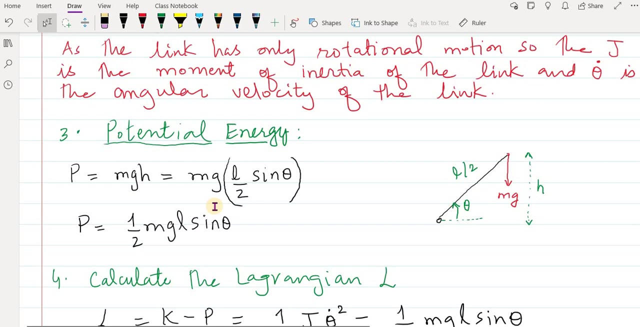 And theta dot is the angular Velocity of the link. So just put the values of j And theta dot and this, You get the kinetic energy of this Robotic manipulator. The third step is to Find the to calculate the Potential energy of your, Of this link. We know that potential energy. 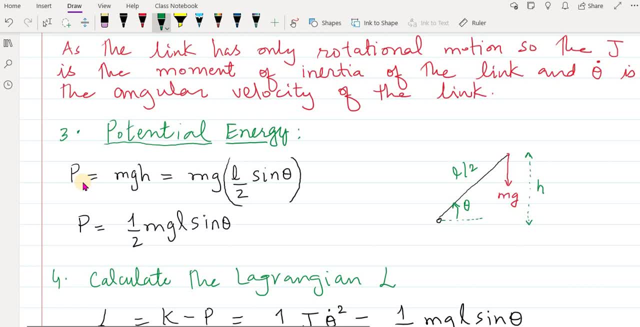 Is equal to mgh. So in this case, If you see the free body diagram Of this link, You see that This is your Center of mass Here And this length is L by 2 Because the center of mass is On the middle of the link. So this force is acting downward. 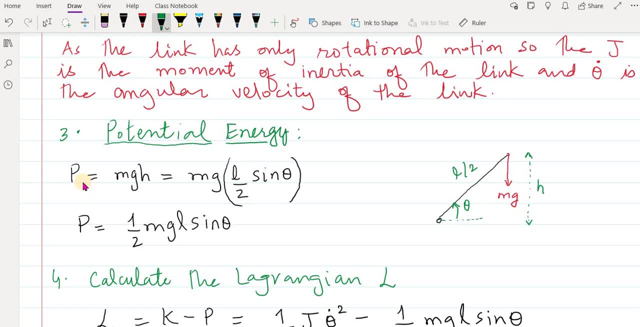 We have angle, theta And what we are interested in. We have the mass, We have the gravity- They are constant- And the value of h, This is a variable. this is changing Because, as the link moves, Rotates, This h will become Bigger or smaller. Okay, So how to calculate the h? 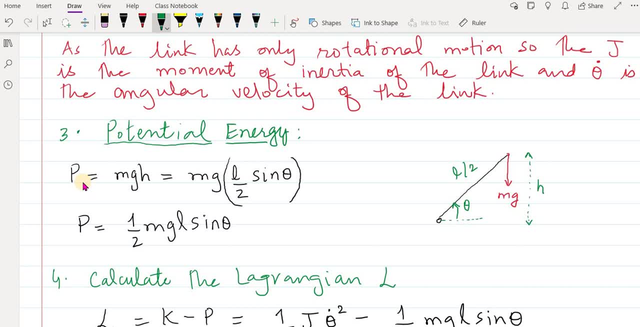 We can. We can solve this Using this right angle triangle. Here, Let's say, h is a perpendicular And we also have the, The hypotenuse of this Triangle, and What you need to do is: We know that the We can find the h, Which is The l, by 2. 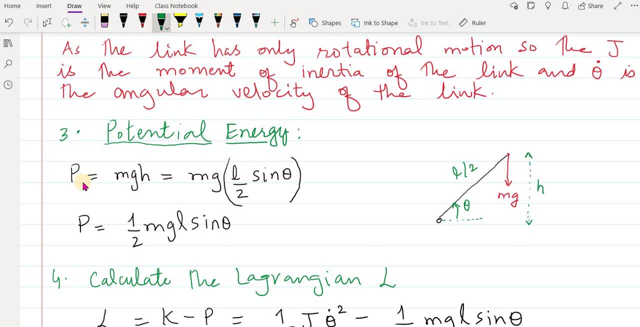 We can multiply this with the, With the sine theta. Okay, So that's what we did here. So instead of h, we have put L by 2 into sine theta. So that's how we have Converted the, This length into This height. Or you can say that We have converted the length and the angle. 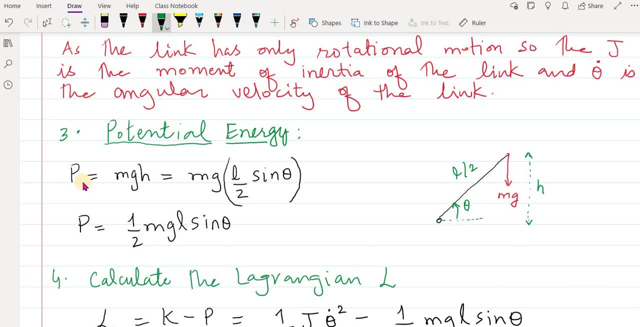 To the height, Or the other way around. we have converted The height into Length and theta And finally we get the potential energy, Which is equal to 1 by 2 mgl Sine theta. So this is the potential energy. Now we have Calculated the kinetic and potential energies. 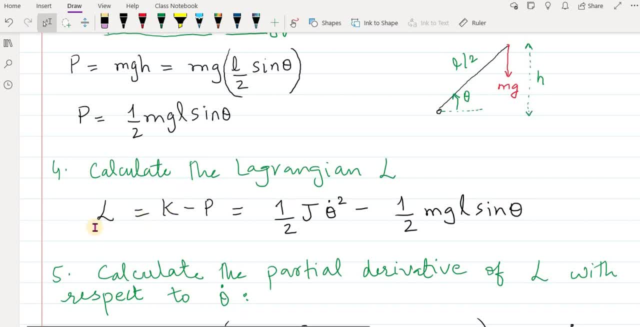 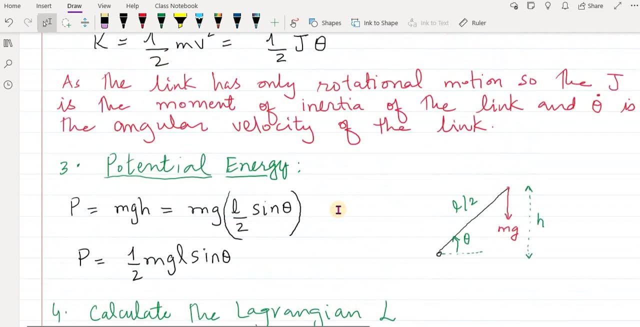 Now we calculate the Lagrangian. We know that this is equal to. Lagrangian is equal to k minus p. Just take the difference of these two terms: 1 by 2 j theta dot square Minus 1 by 2 mgl sine theta. 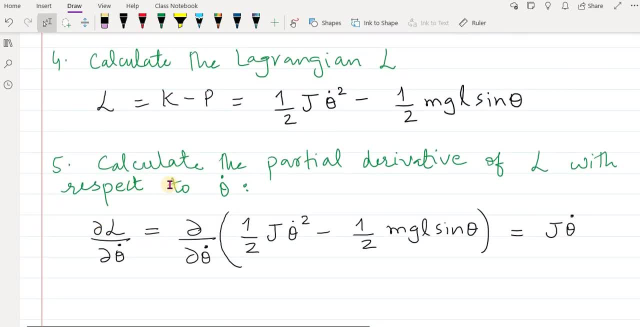 So now you have the Lagrangian Also Calculate the partial derivative of Lagrangian With respect to theta dot. So we take its partial derivative of this Term here With respect to theta dot. With respect to velocity, When we take the partial derivative This term, When the 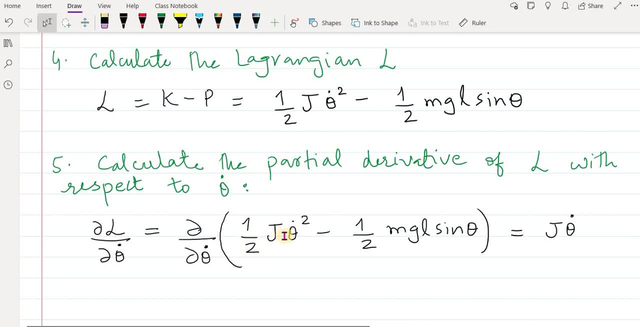 This is constant j and 1 by 2 Is constant And we take the derivative of theta dot. square 2 will come here Down, multiply And it will Cancel by this 2 And then we have only theta dot. So We have only j theta dot here. 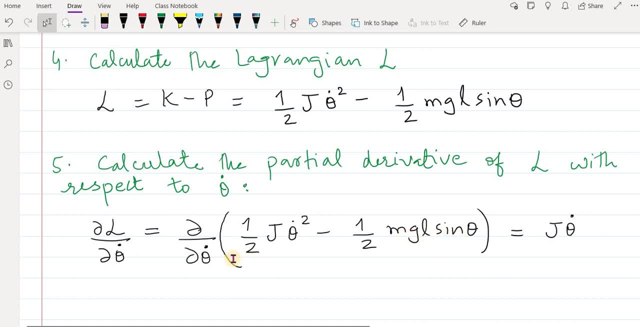 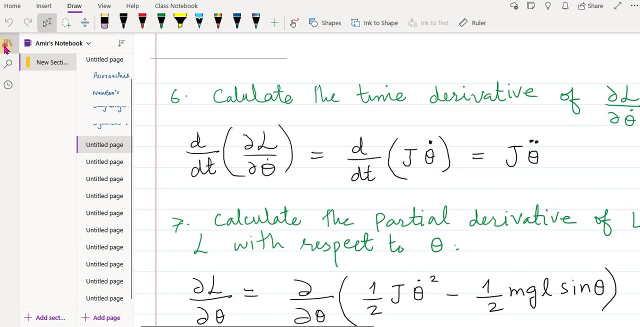 And then we have the second term. These all are constant with respect to theta dot. Okay, and then this Term will become zero And the answer will be j theta dot. The next step is to. Next step is to calculate the Time derivative of This term that we have calculated. 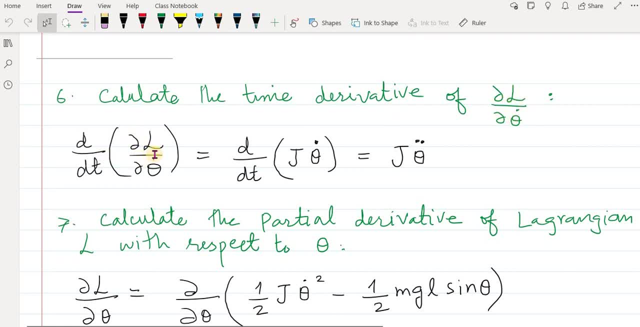 In the step 5. So We have calculated this term here, Which was j theta dot. We take the time derivative of this, And the time derivative of This variable Can be shown as theta double dot. Okay, this is a Constant. it will remain like this And the final answer will be: 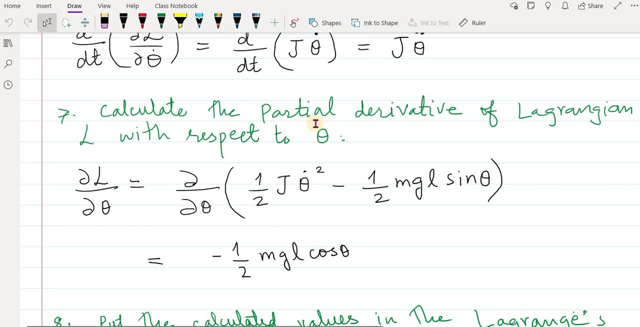 j theta double dot. Calculate the partial derivative Of Lagrangian With respect to theta. So now again, We have a Lagrangian and We take its partial derivative with respect to theta. So in this case this term Will become zero because they are all Constant with respect to. 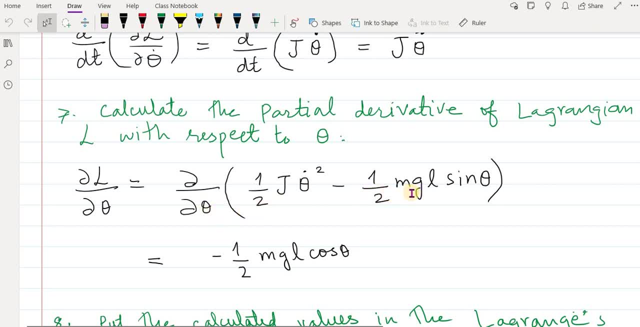 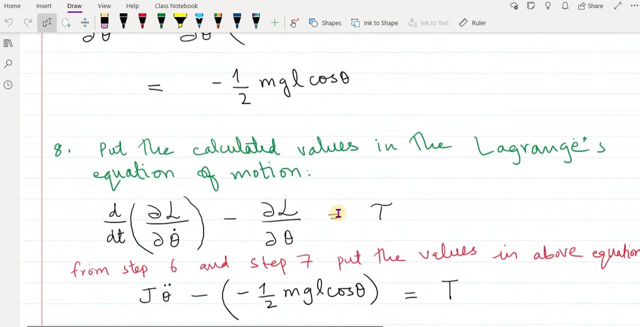 Position And this term will be. This is constant and This is a variable And if you take the derivative of A sine theta, it will be Cosine theta. So your final answer will be Minus 1 by 2 MGL cosine theta And in the Step 8: 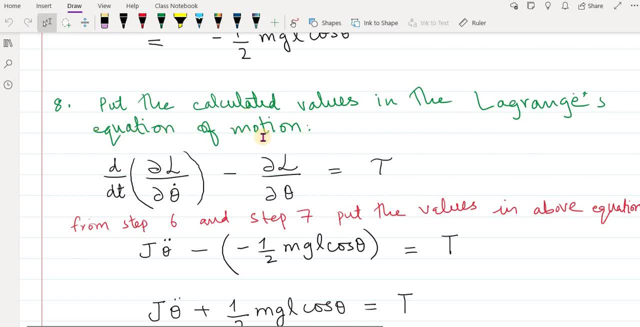 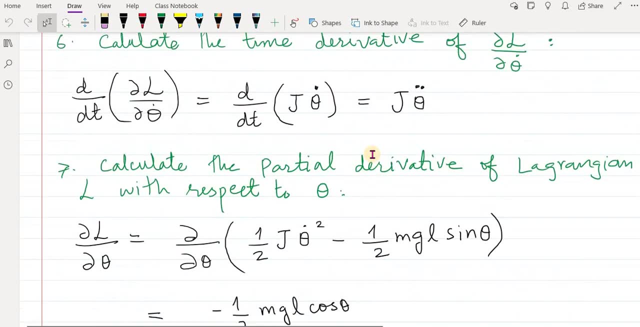 We put the calculated values in the Lagrangian equation of motion. We know that this was a Lagrangian equation Of motion and you Just have calculated the values In the previous steps. You just have to put the values. So, from step 6 and step 7. 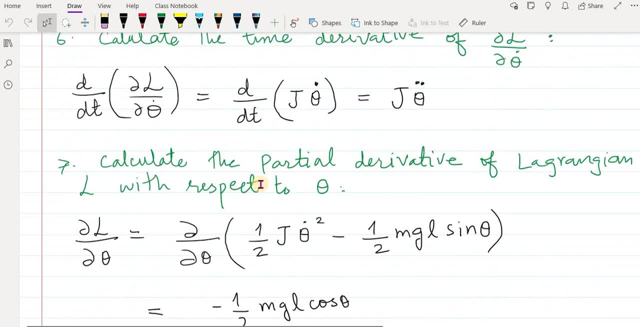 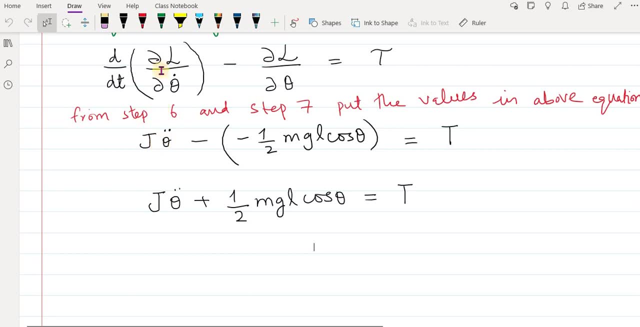 Put the values in above equation. So Step 6 says that This term is equal to j theta double dot. We put here j theta double dot. here, In this term, you have put here j theta double dot And for, In place of this term, We have put this: